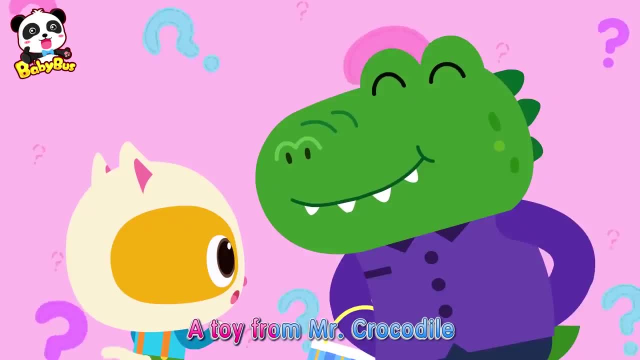 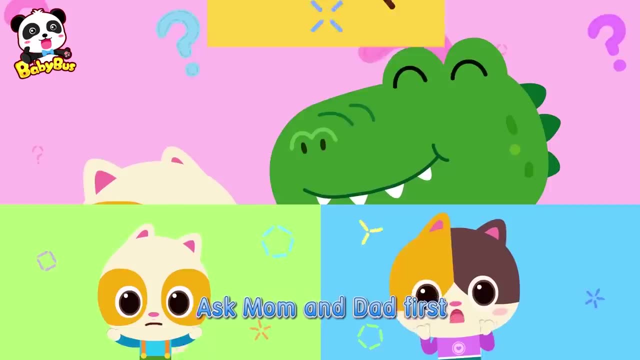 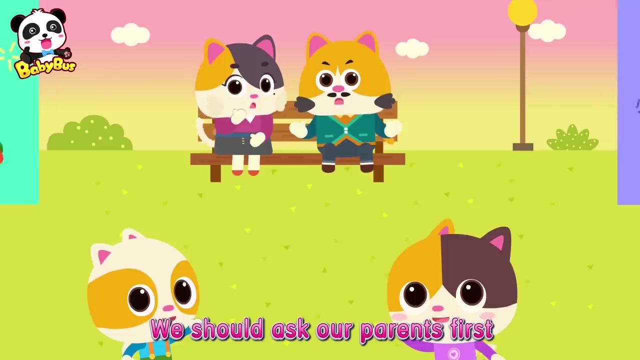 Can I take it or not? A toy from Mr Crocodile: Can I take it or not? No, no, no, no, no, no. Ask Mom and Dad first. Even if we know them, We should ask our parents first. Can we take one thing? 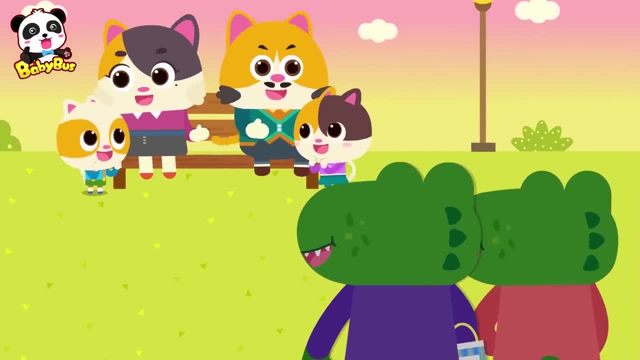 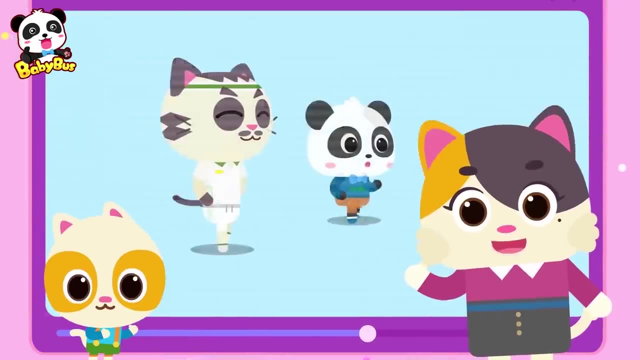 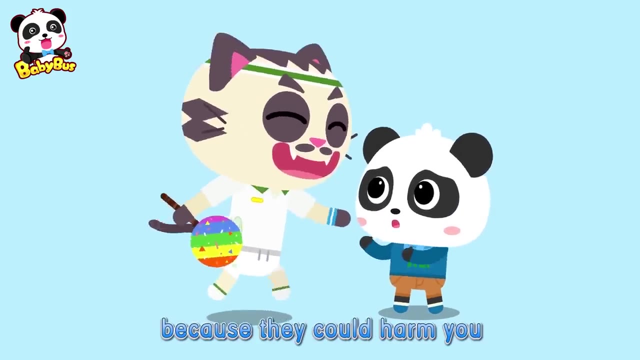 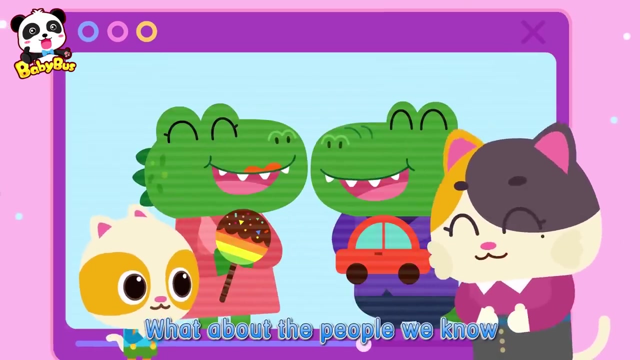 Can we take one? Can we take one? Yay, Thank you. Don't take anything from strangers, No matter how much you want it, And stay away from them Because they could harm you. What about the people we know? Always ask Mom and Dad first. 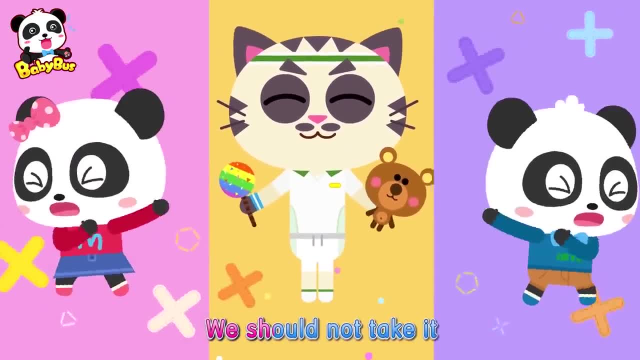 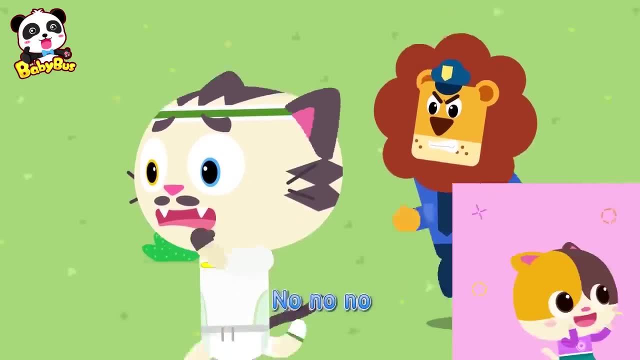 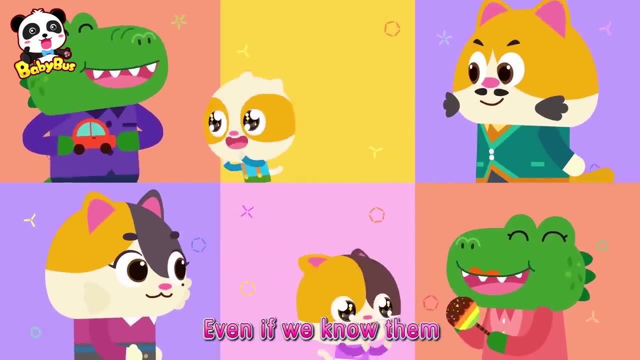 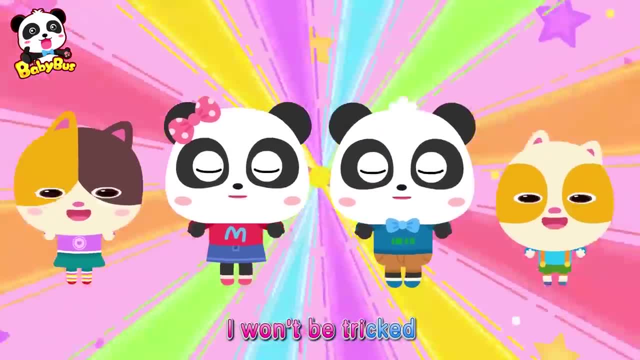 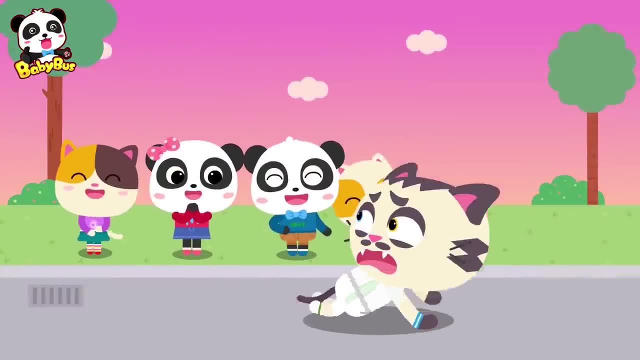 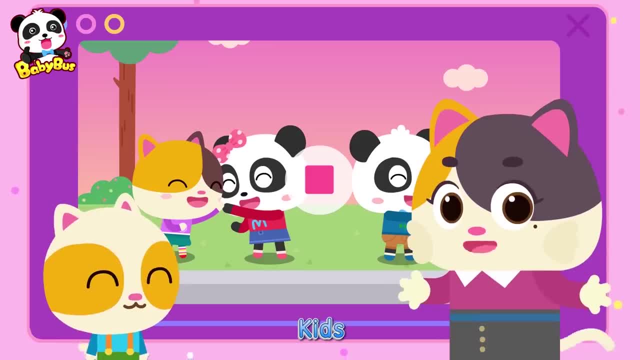 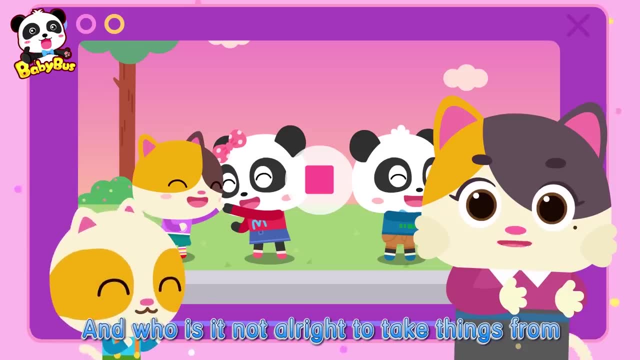 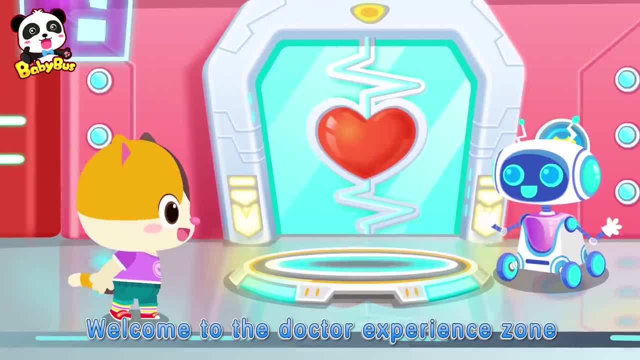 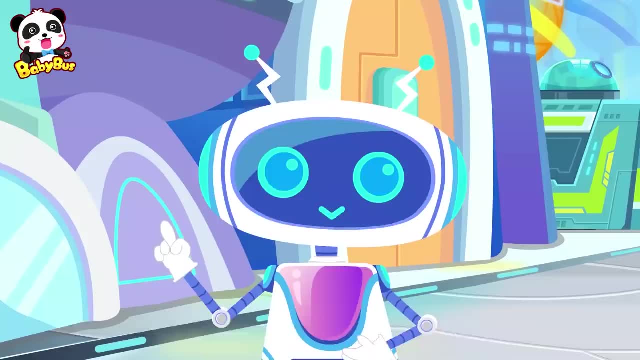 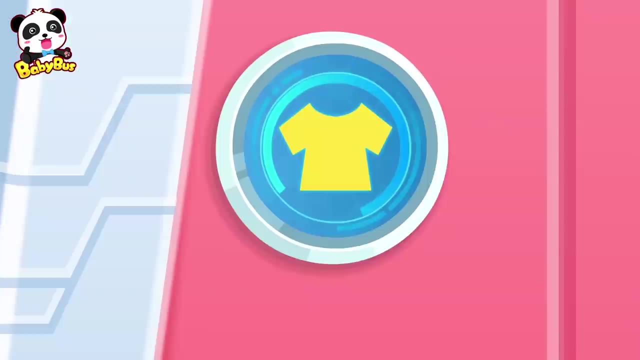 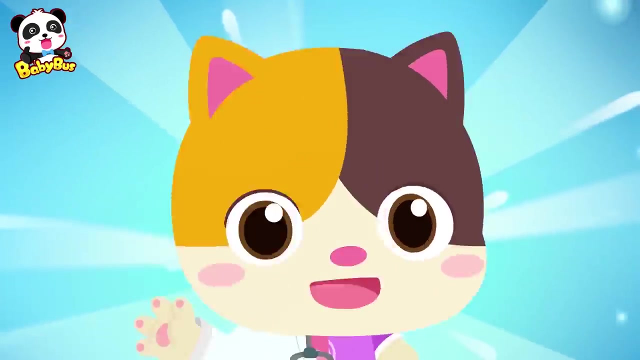 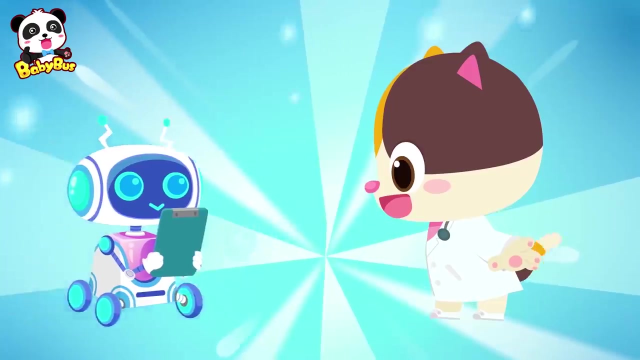 Which dog should I choose? Welcome to the Doctor Experience Zone, Doctor. Wait, Mimi, You need to change into your uniform first. Okay, Sorry, I forgot Time to change. Woohoo, I'm Dr Mimi. Doctors wear white coats over their own clothes. 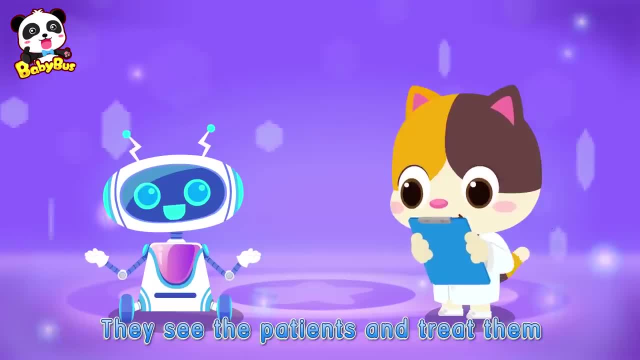 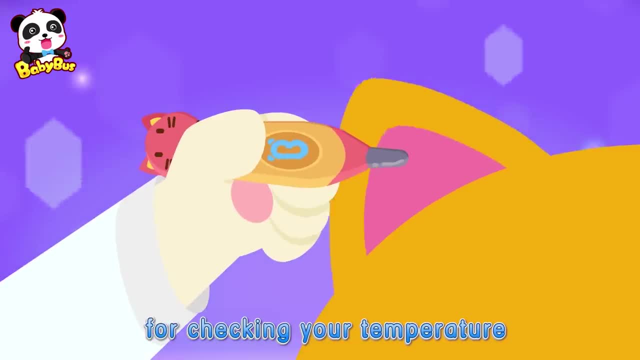 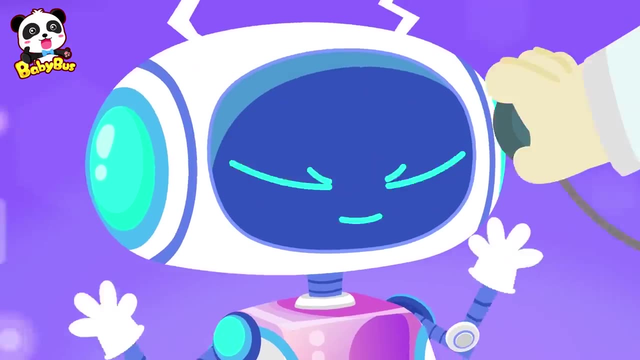 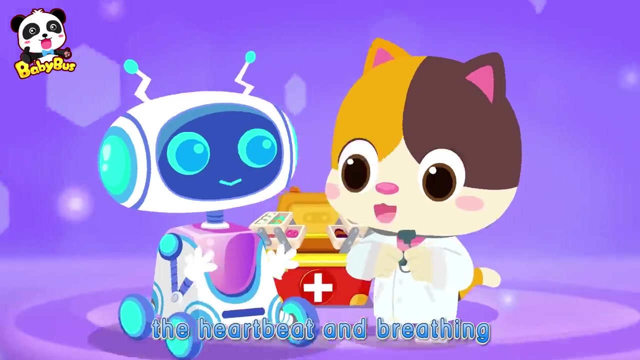 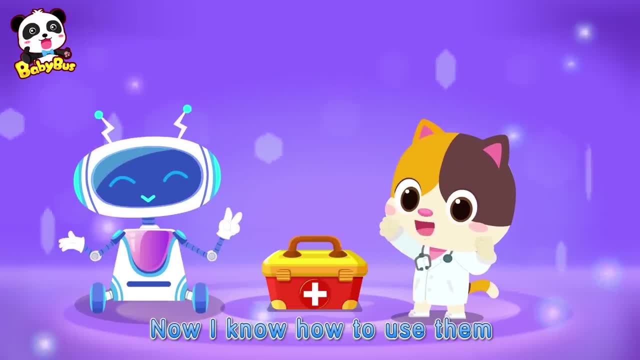 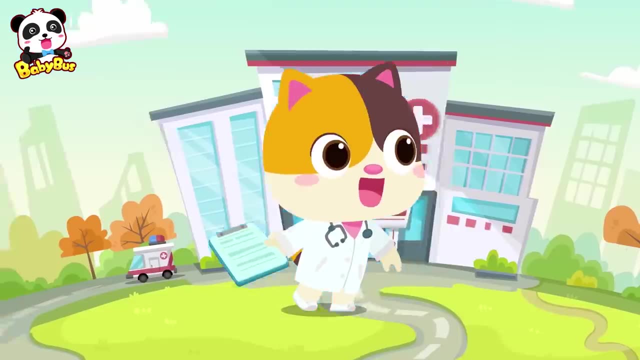 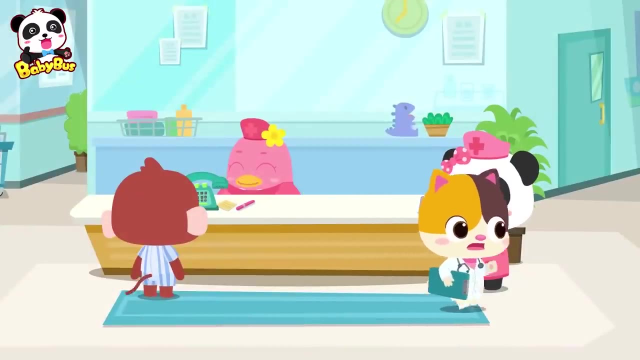 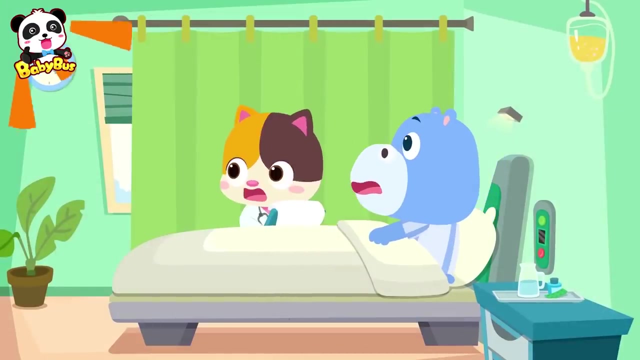 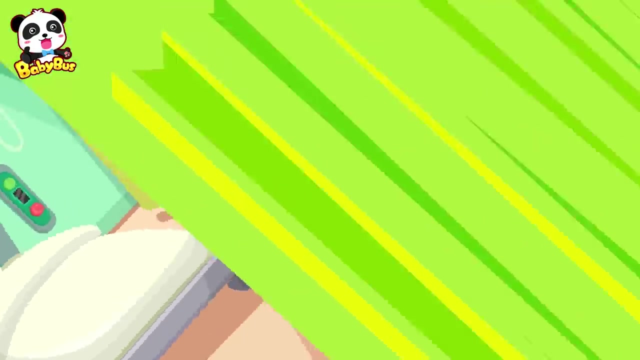 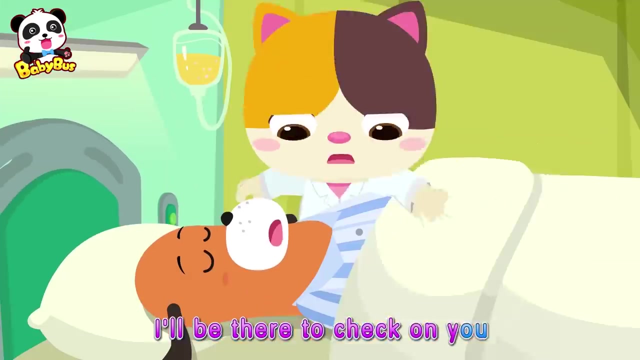 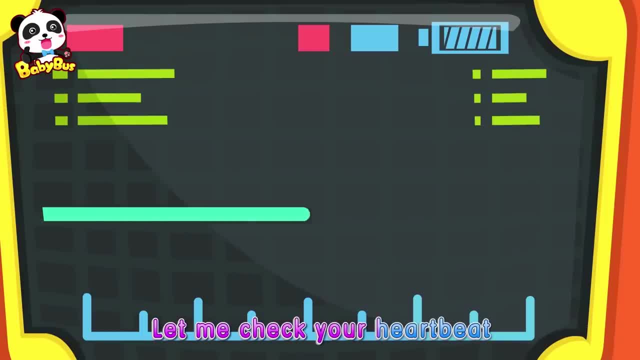 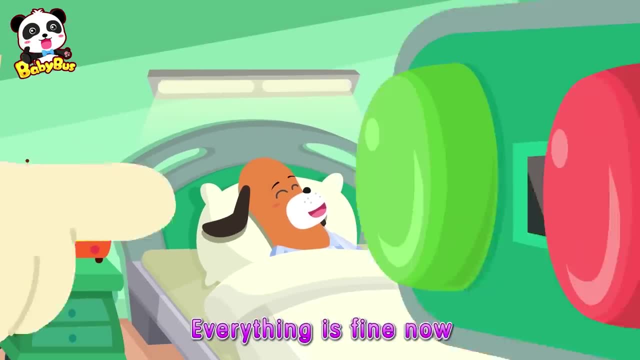 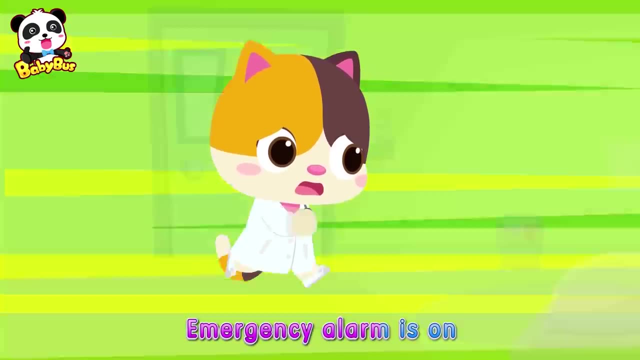 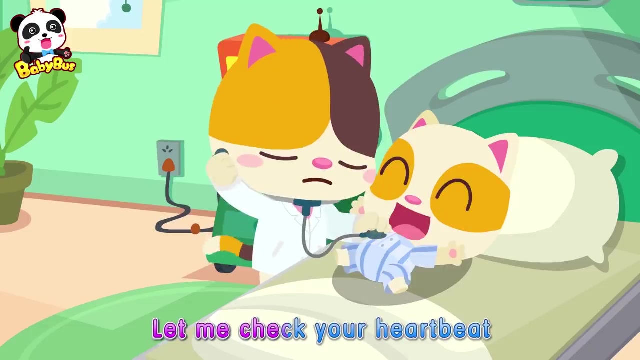 Go, go, Emergency, let me check your heartbeat. Thump thump, thump thump. Everything is fine. now Emergency alarm is on. I'll be there to check on you. Go, go, Emergency. let me check your heartbeat. Don't worry, you'll be okay. 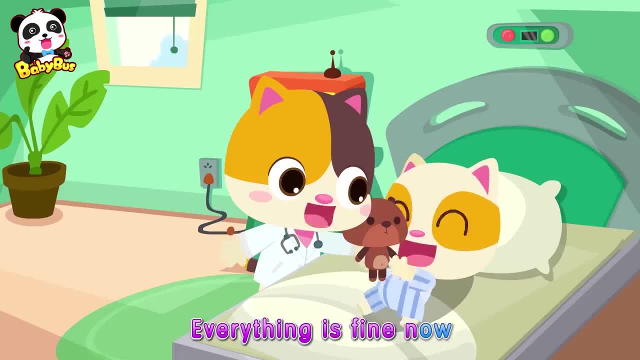 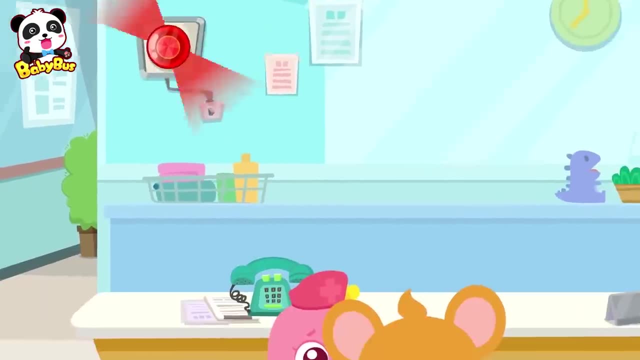 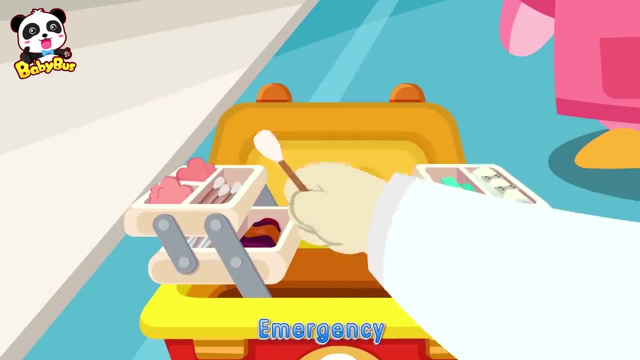 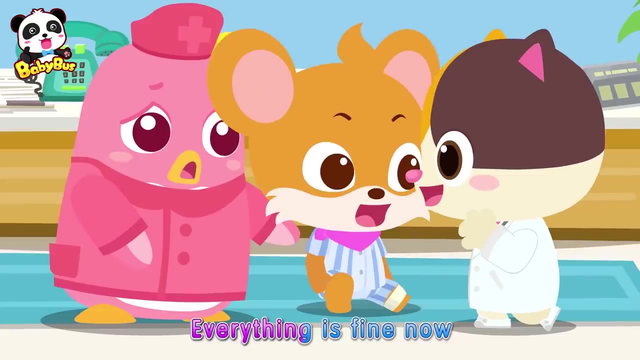 Everything is fine now. Don't push the alarm button just for fun. Uh-huh, Emergency alarm is on. I'll be there to check on you. Go, go, Emergency. let me treat your wound And bandage up your leg. Everything is fine now. The parlor gap. 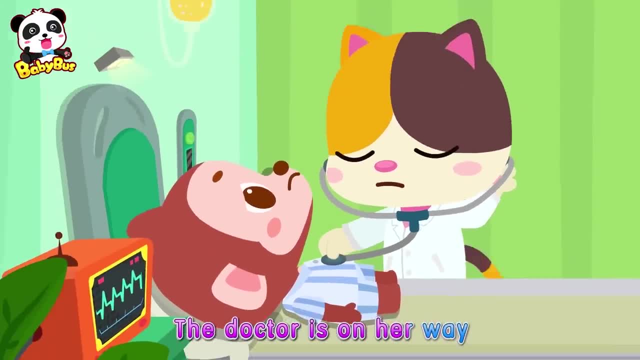 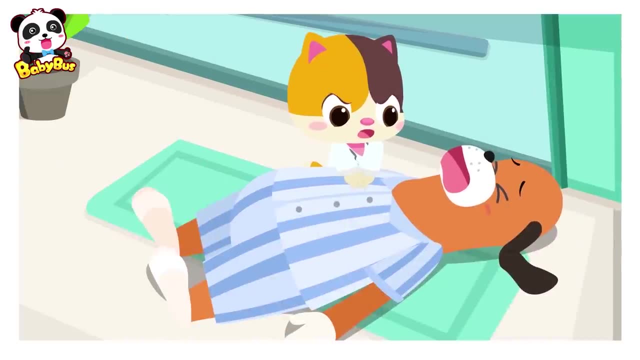 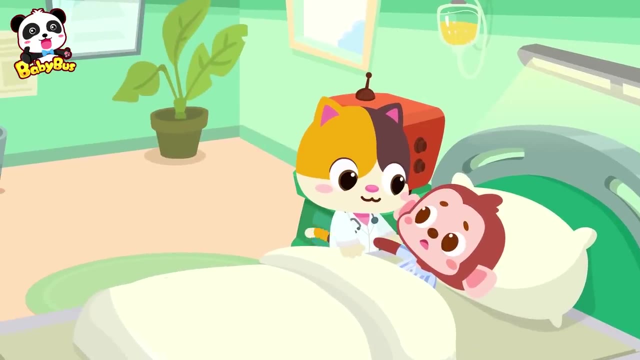 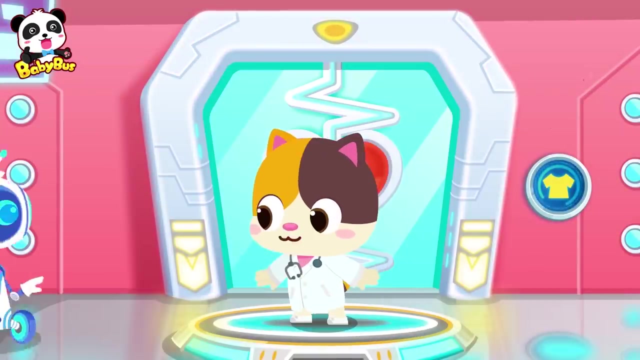 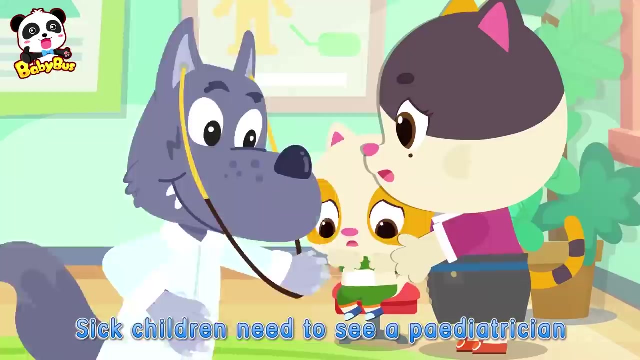 Is open Emergency. The doctor is on her way, Everything is fine now. You're fine. now Get some rest. I had so much fun. Did you know that there are different kinds of doctors? Sick children need to see a pediatrician. When you need to check your teeth? 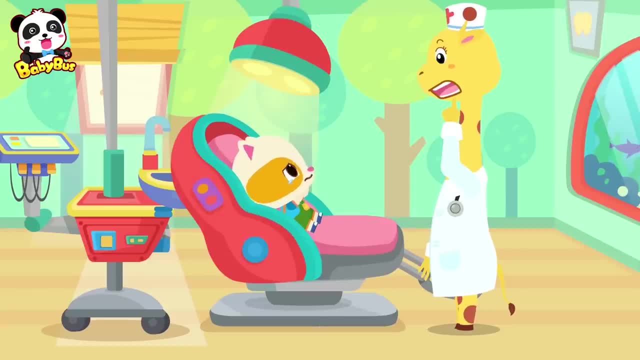 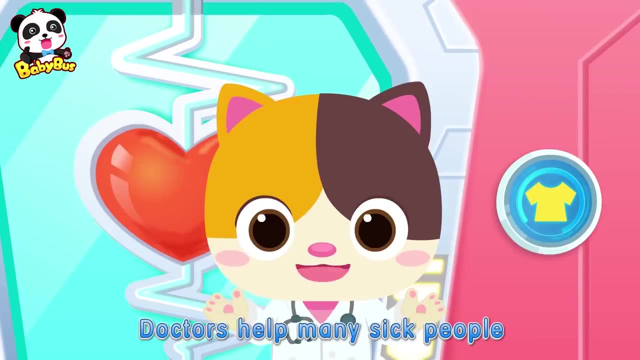 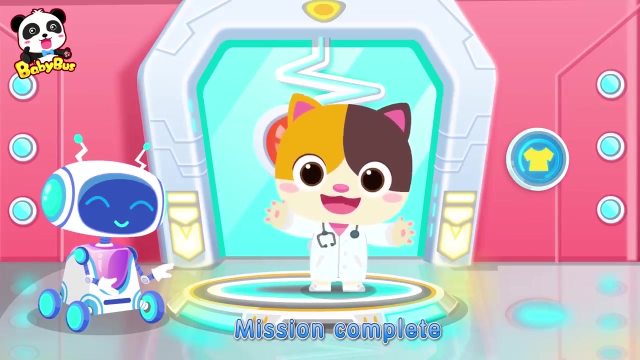 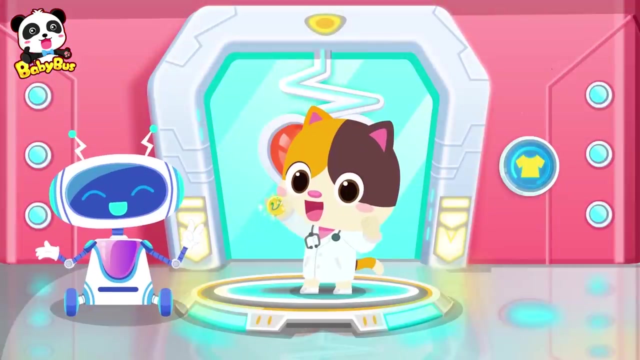 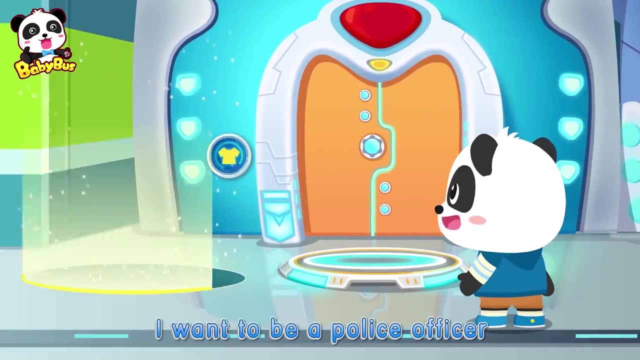 You see a dentist When you have problems in your eyes, You see an ophthalmologist. Doctors help many sick people. That's great. Yeah. One day doctor mission complete, You've got a doctor badge. Yay, Wow, I want to be a police officer. Ding ding. 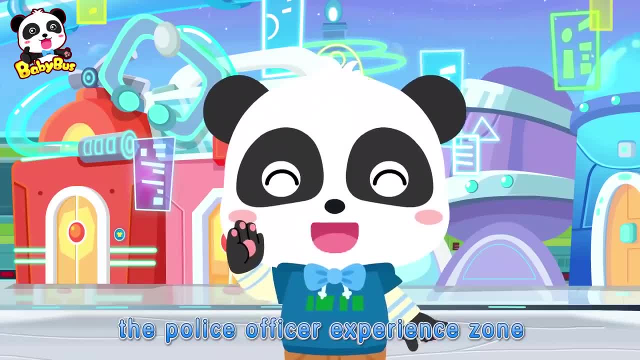 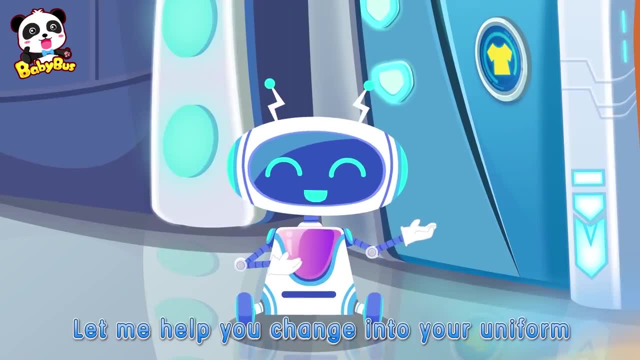 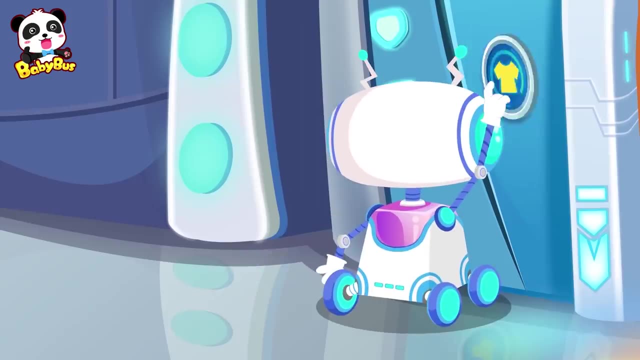 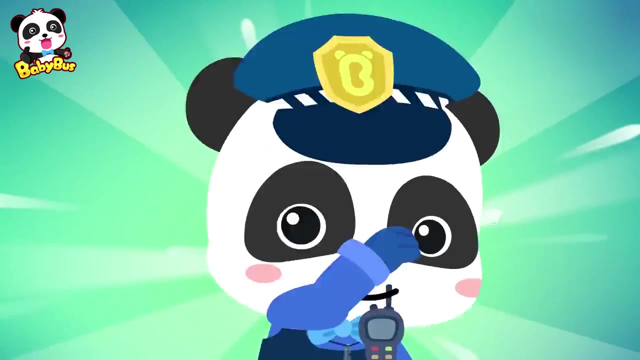 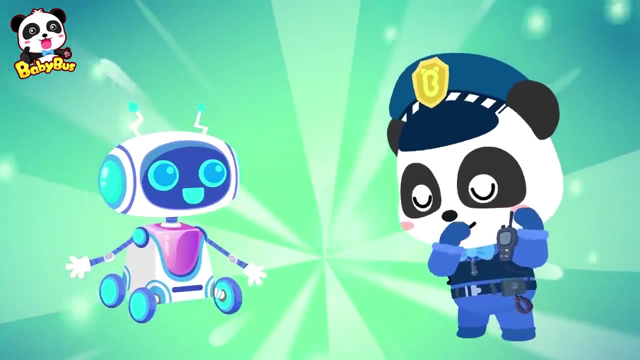 Welcome to the police officer experience zone. Officer Kiki is here. Hi, Officer Kiki, Let me help you change into your uniform. Okay, Wow, I'm a police officer. What I'm a police officer? Huh, Time to change. I'm Officer Kiki. How do I look? 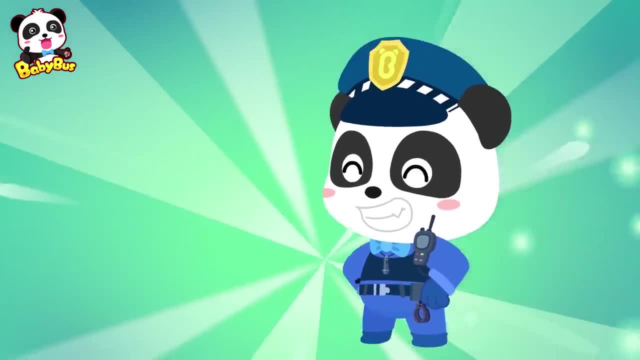 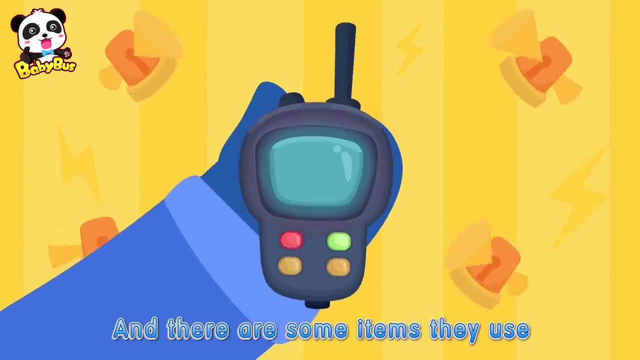 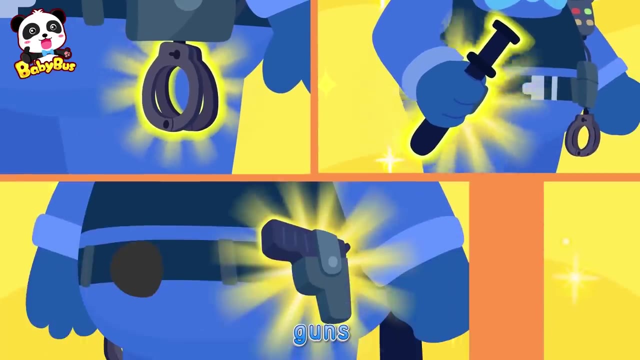 Do I look cool in uniform? Of course, Officer Kiki. Police officers wear uniforms with caps while on duty, And there are some items they use. Radios are used to communicate with police officers with each other, and there are handcuffs, batons, guns and whistles. they are used when police. 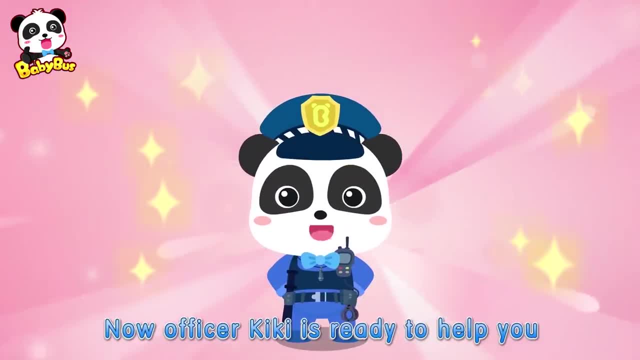 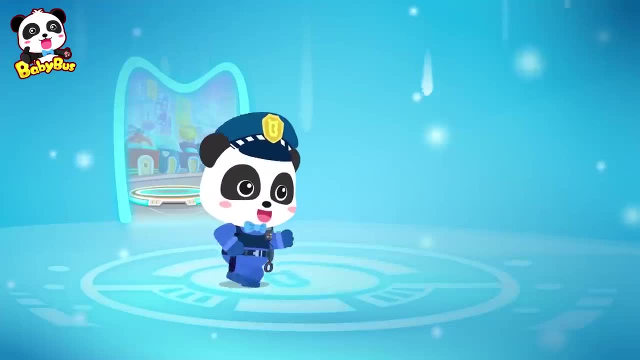 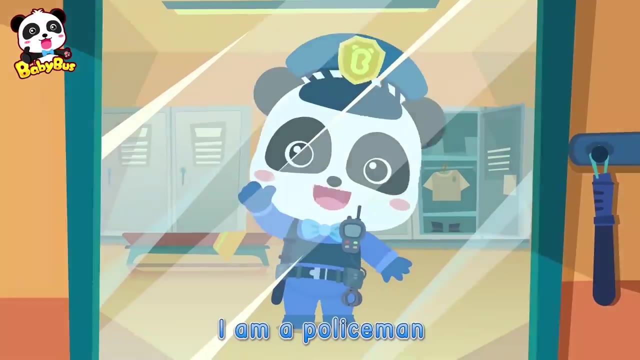 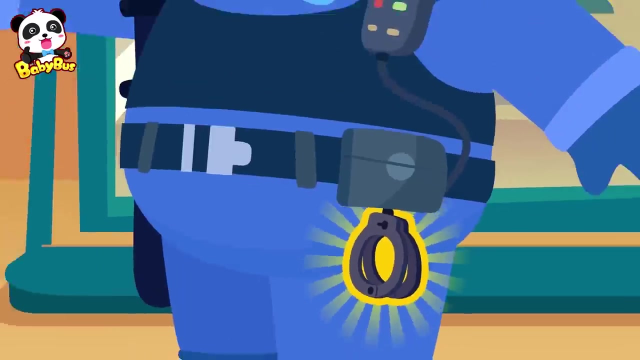 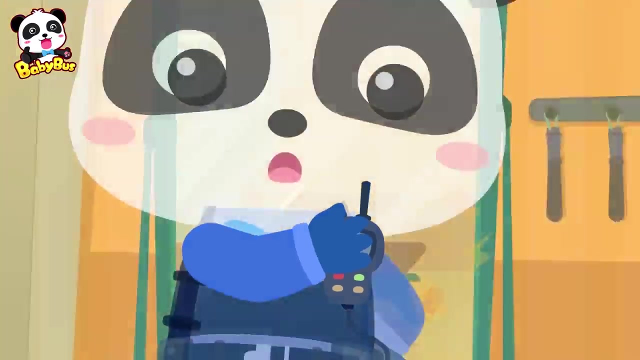 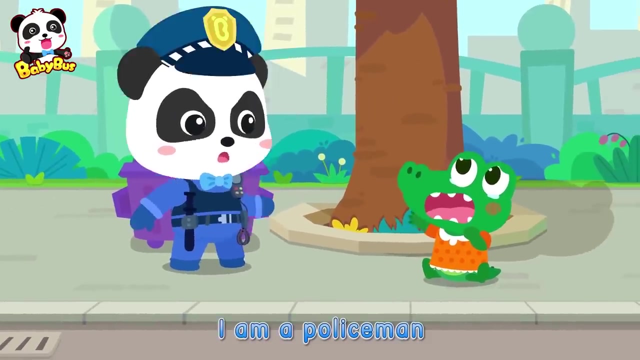 officers catch bad guys. now, officer kiki is ready to help you one day. police officer, let's start. oh, wow, i am a policeman in a cool uniform with police equipment. wow, i'm the best policeman. yeah, i am a policeman keeping people safe and sound. call me when you're in trouble. 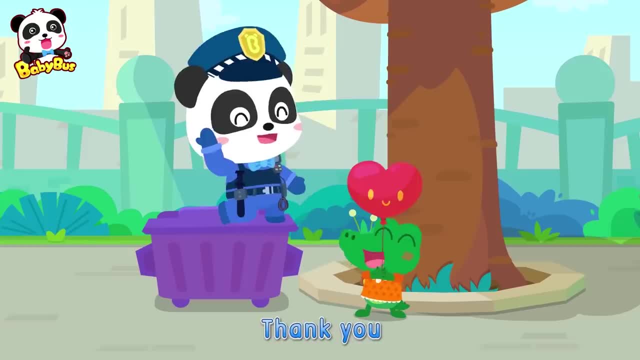 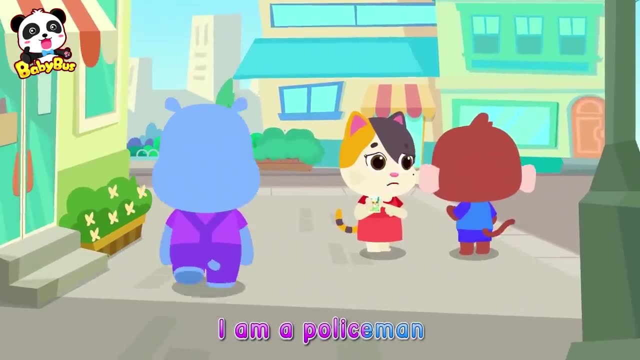 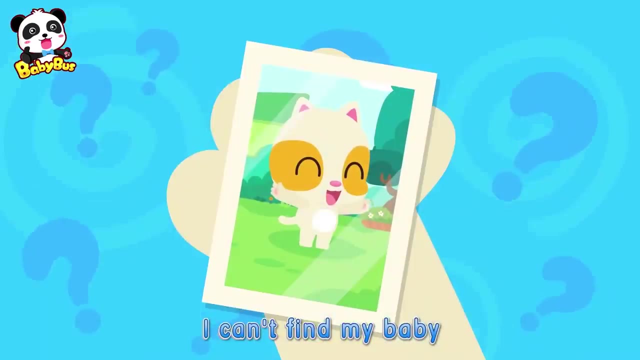 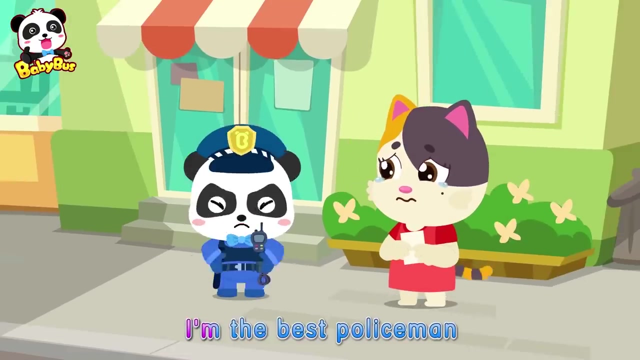 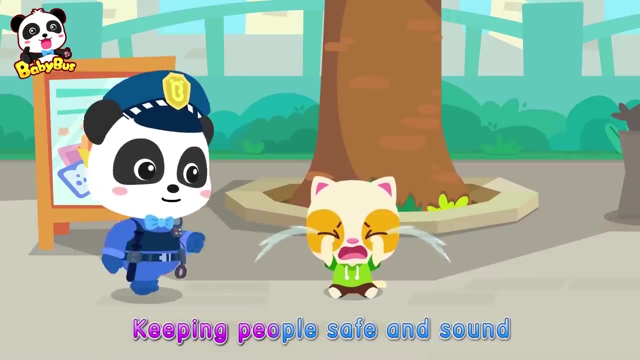 aha, thank you, i'm the best policeman. i am a policeman keeping people safe and sound. call me when you're in trouble. my baby, i can't find my baby, don't worry, i'm the best policeman. i am a policeman, keeping people safe and sound. call me when you're in trouble. 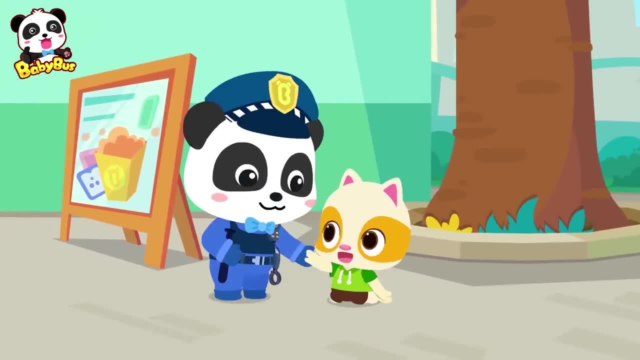 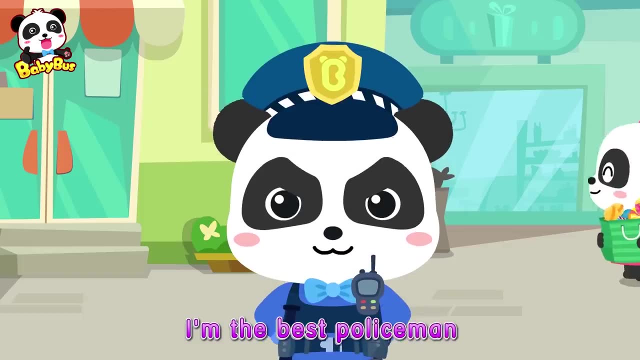 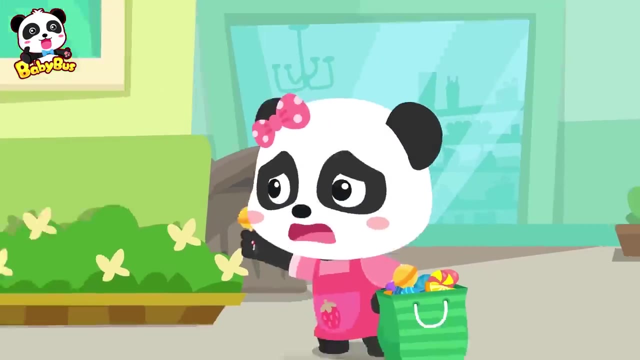 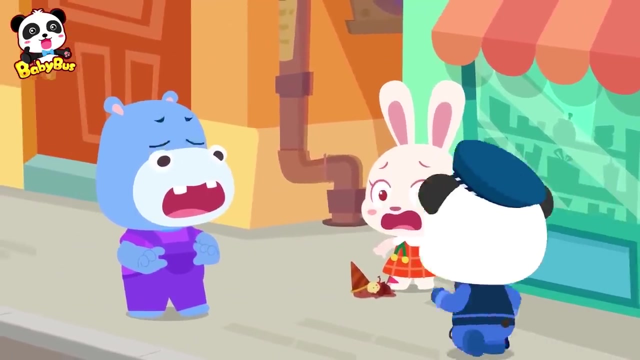 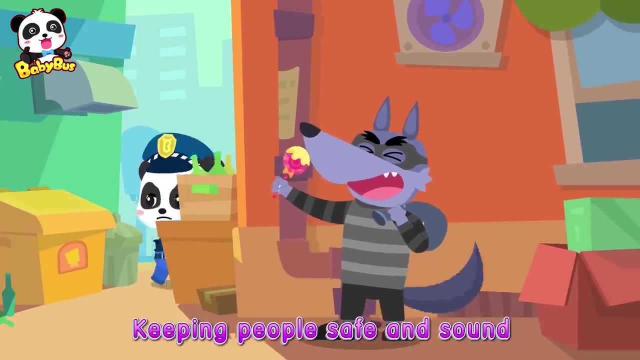 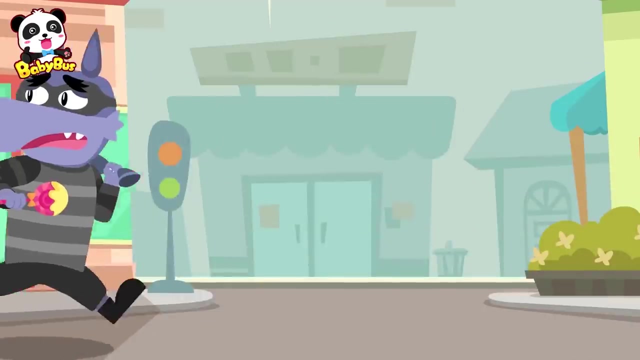 i'll take you to your mom, sweetie. thank you, policeman. i'm the best policeman. leave it to me. i am a policeman keeping people safe and sound. call me when you're in trouble. stop right there. i got you. i'm the best policeman. leave it to me quickly. 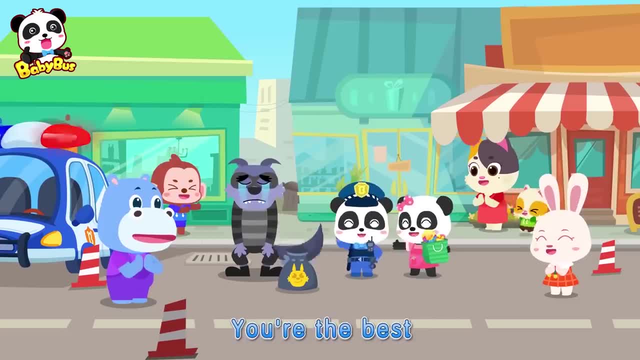 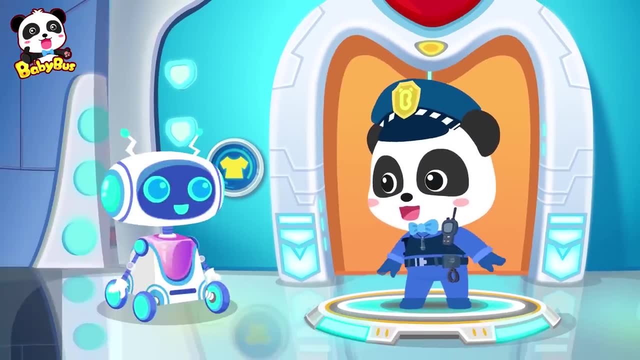 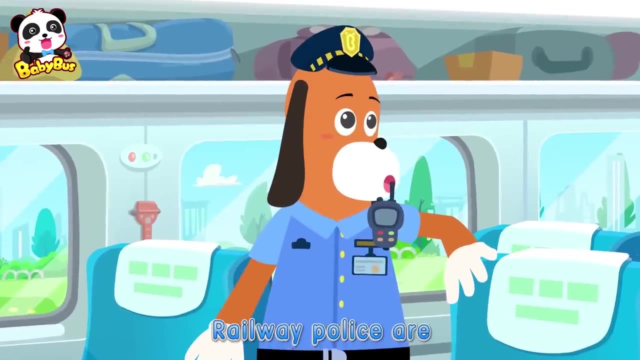 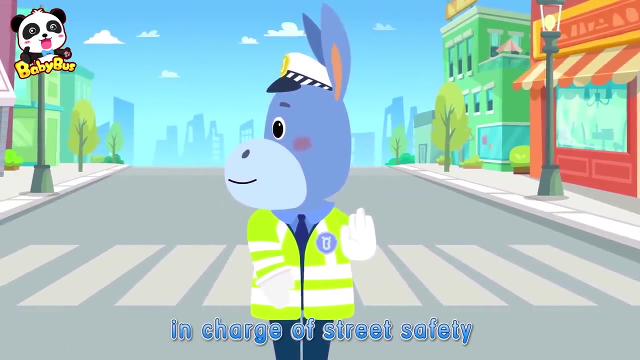 walk slowly. that's what you're fine. yeah, Take that. hey, Wow, That was a good break. you're the best. you're the best. I had so much fun. there are different types of police who do different things. railway police are in charge of train safety. traffic police are in charge of street safety. 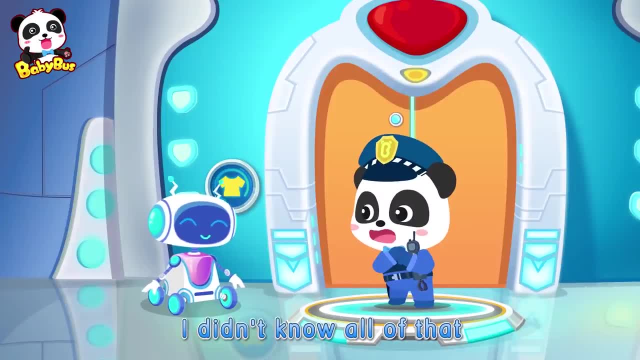 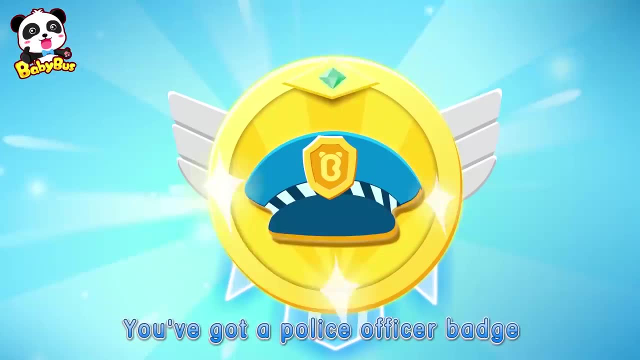 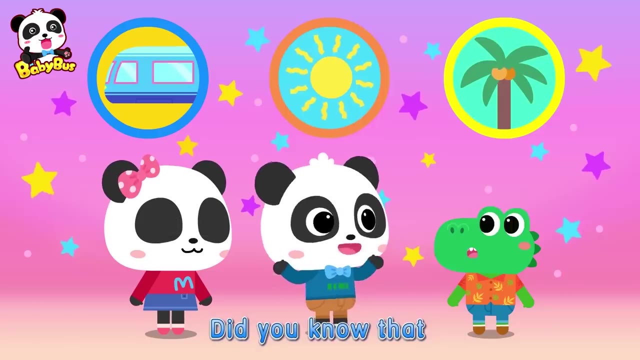 and airplane safety. Whoa, I didn't know. all of that Sounds interesting. One day, police officer mission complete, You've got a police officer badge. Yay, Did you know that we need to keep our private parts safe in public places? 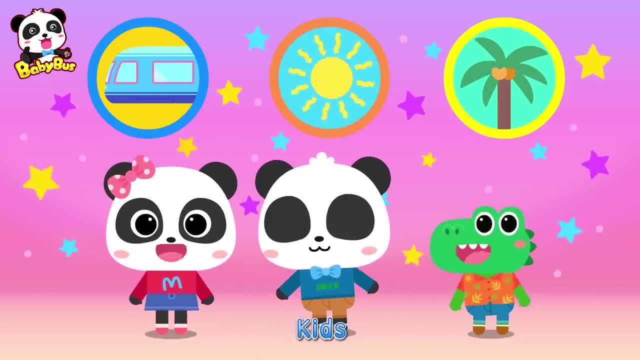 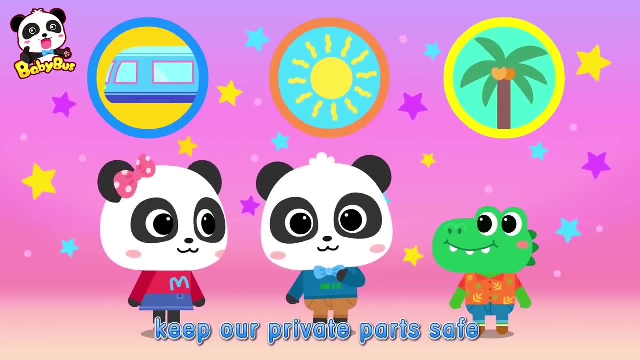 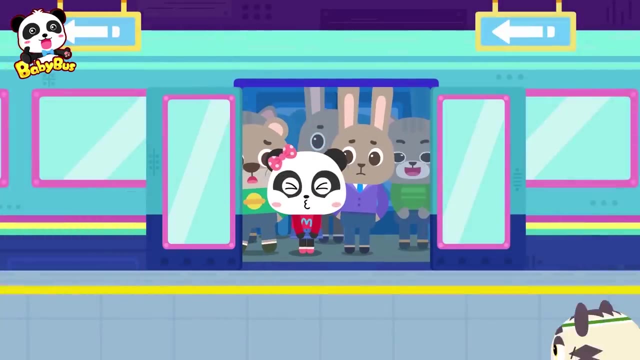 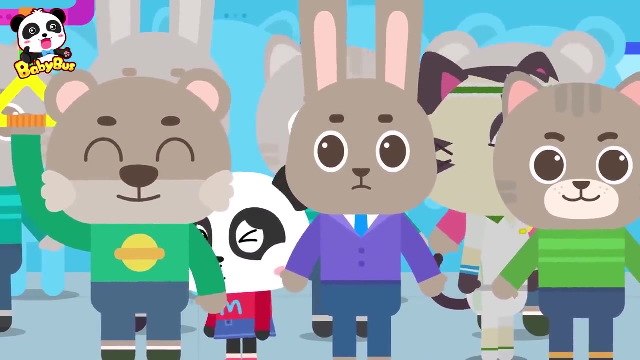 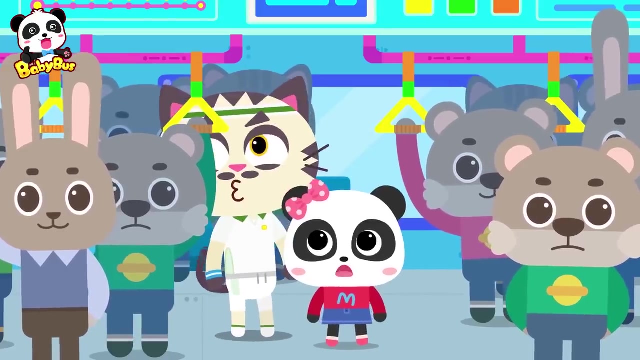 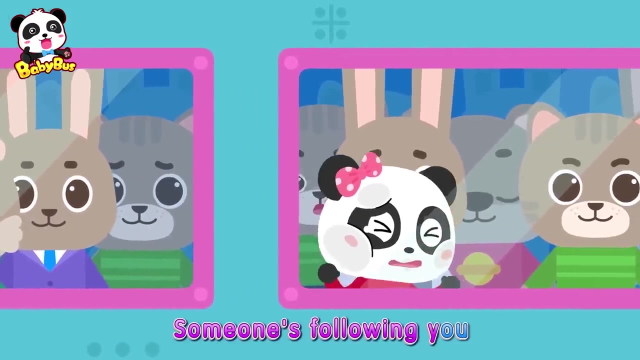 Keep my private parts safe. Yeah, Kids, watch this video with your mom and dad And find out why we have to keep our private parts safe in public places. Someone's following you on the train. Someone's following you on the train. 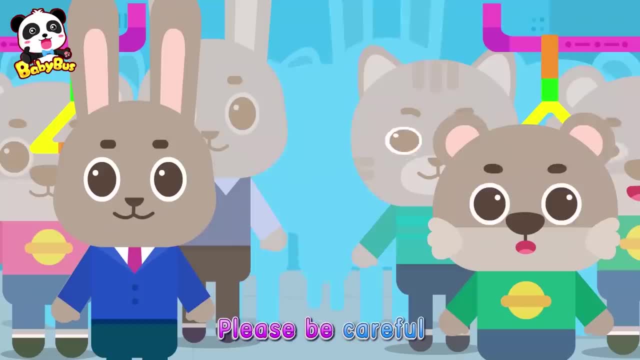 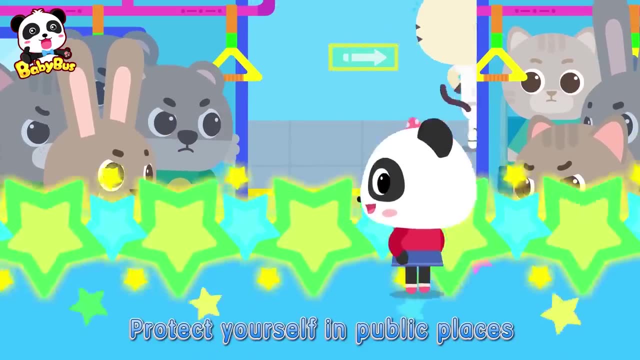 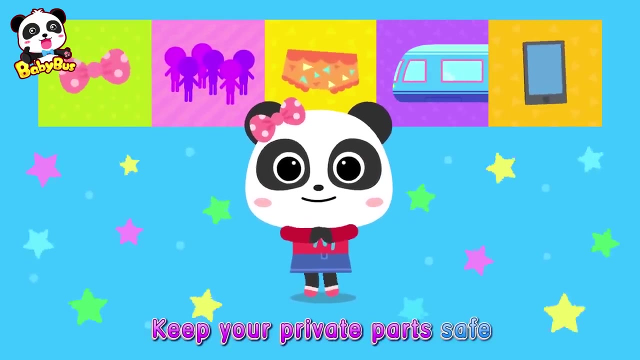 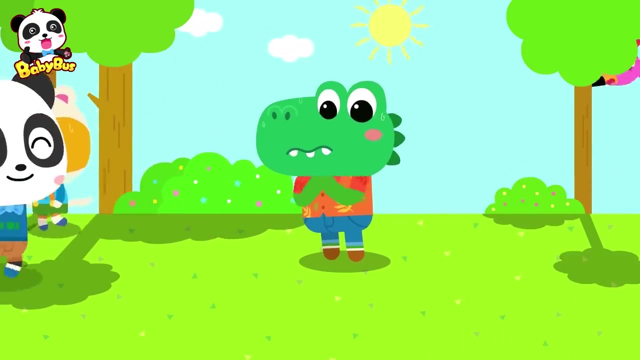 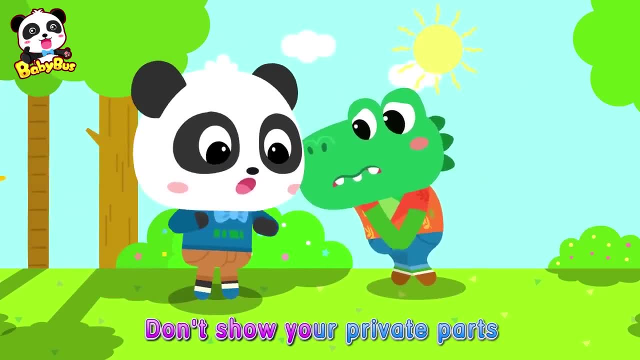 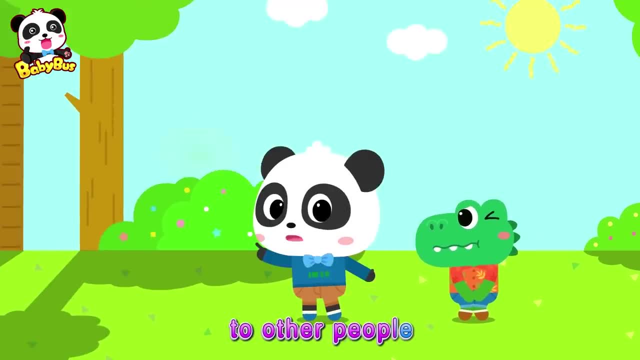 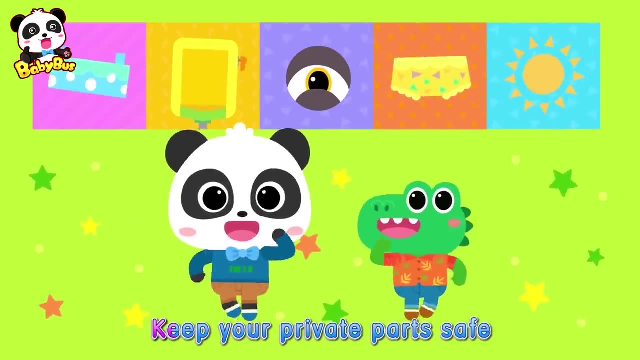 Keep your private parts safe When you change your clothes. be careful. A few hours later, the police officer comes back. Yes, Be careful. Bye-bye, Bye-bye, Bye-bye. Thanks for coming, baby, Bye-bye. 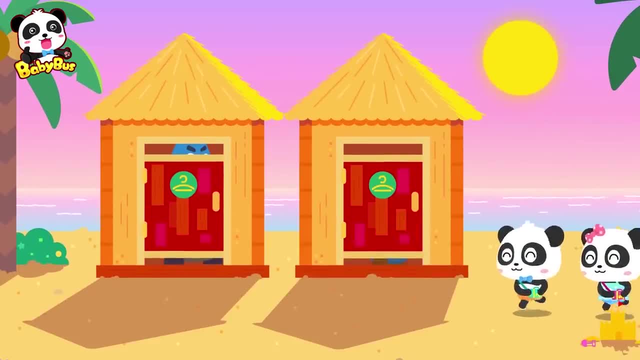 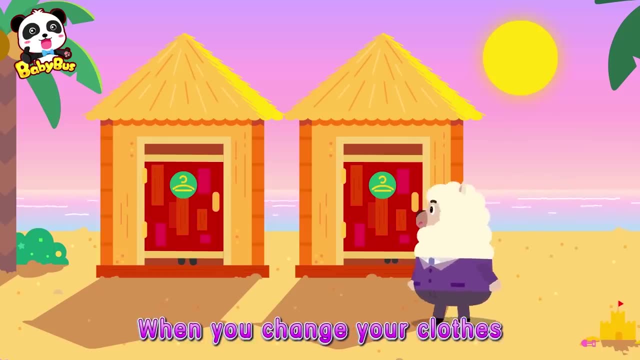 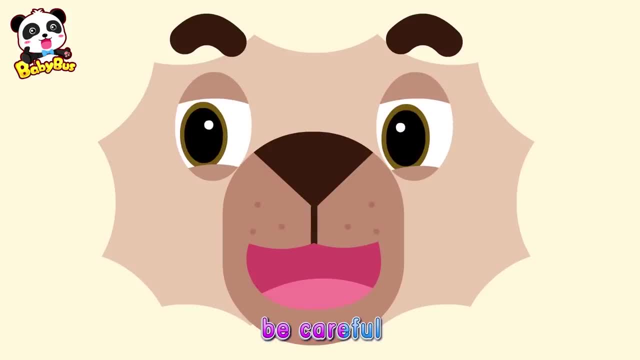 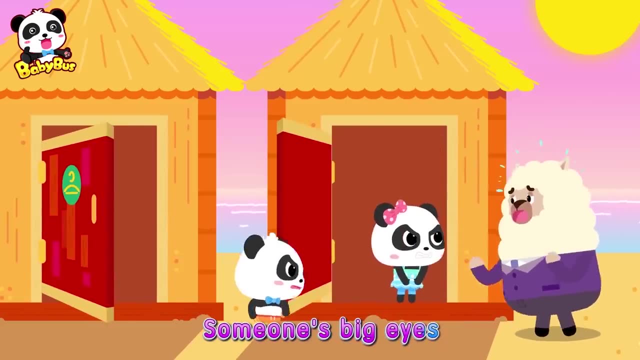 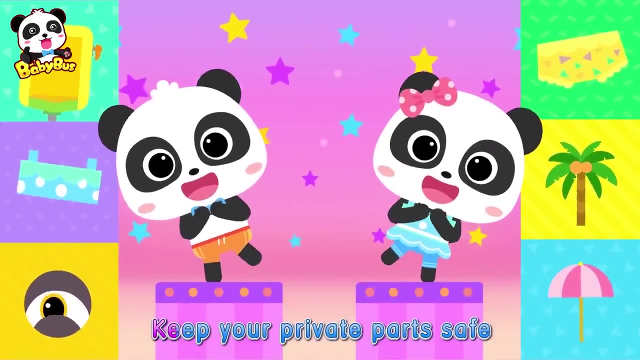 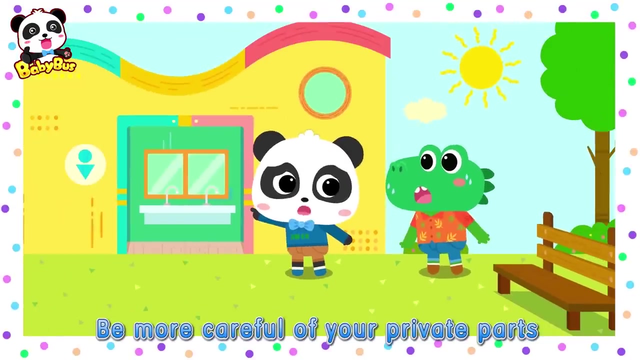 When you change your clothes, be careful. Someone's big eyes might be watching you. Someone's big eyes might be watching you. Protect yourself in public places. Keep your private parts safe. Be more careful of your private parts in public places And don't let others see them. 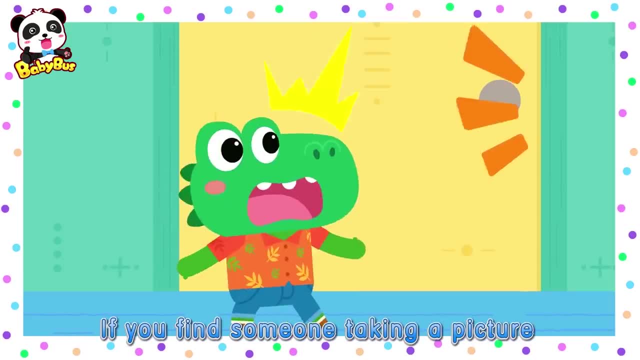 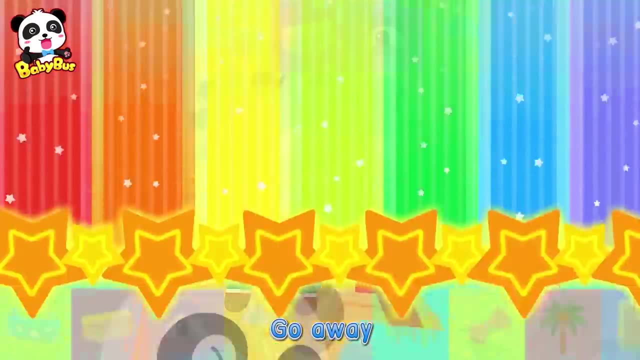 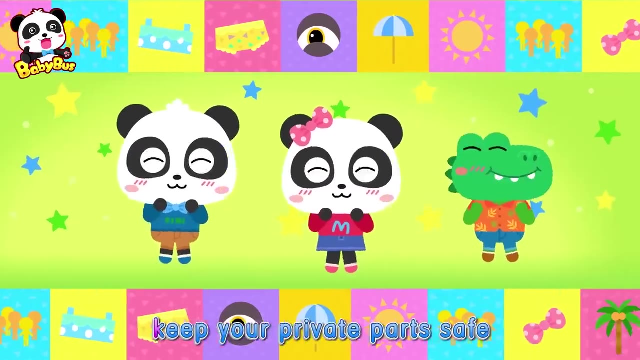 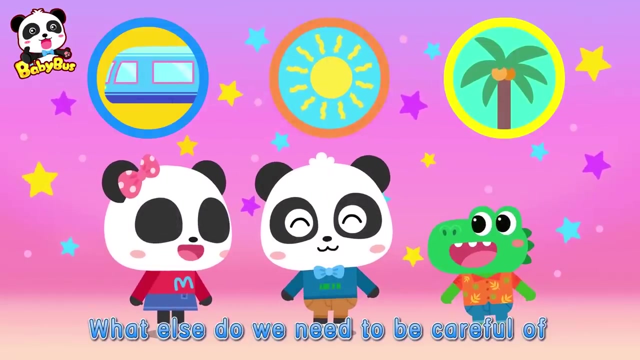 If you find someone taking a picture or peeking at them, Call for help right away. Go away. Protect yourself in public places. You need to keep your private parts safe. What else do we need to be careful of in public places? Now talk about it with your mom and dad. 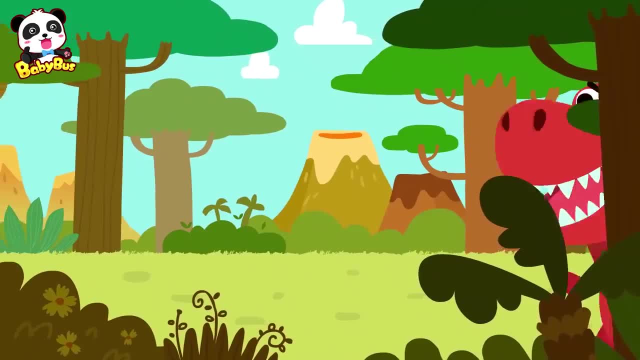 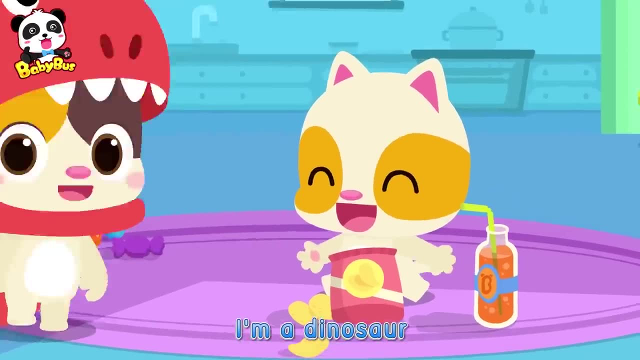 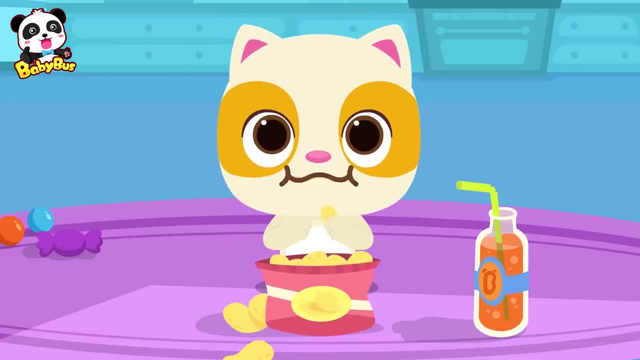 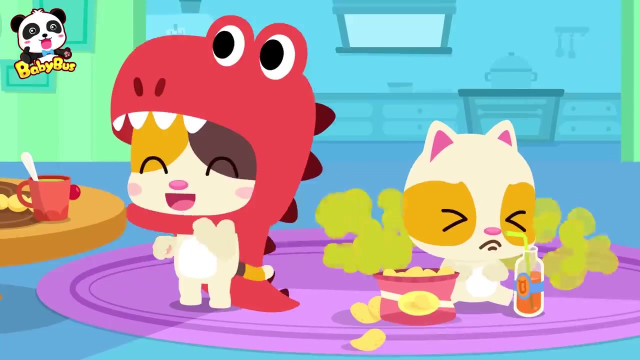 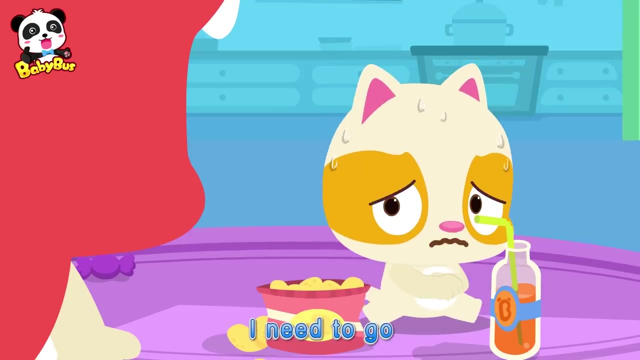 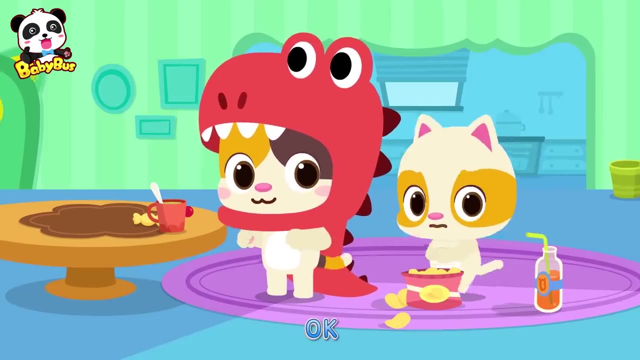 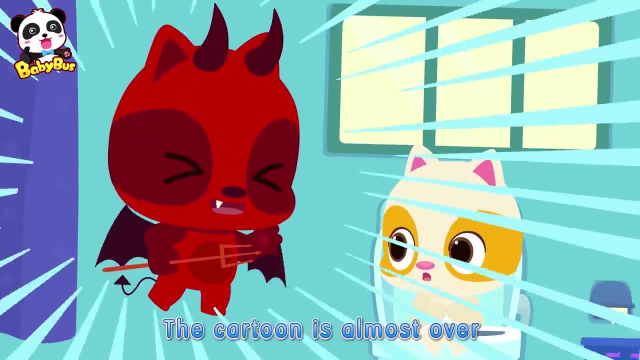 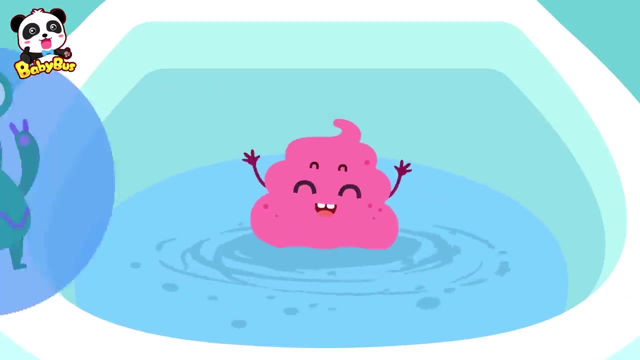 Dad, Okay, I'm a dinosaur. Toonie, that smells really bad. I need to go…. Go to the restroom now. Okay, The cartoon is almost over. I can't miss the ending. Let's go right now. Let's go right now. Let's go right now. 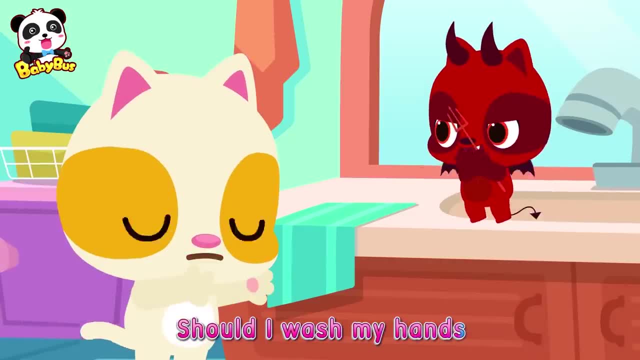 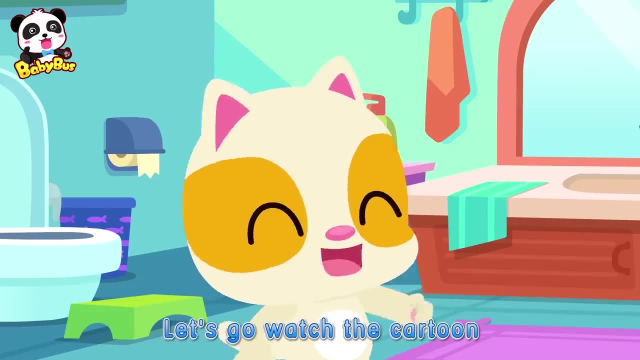 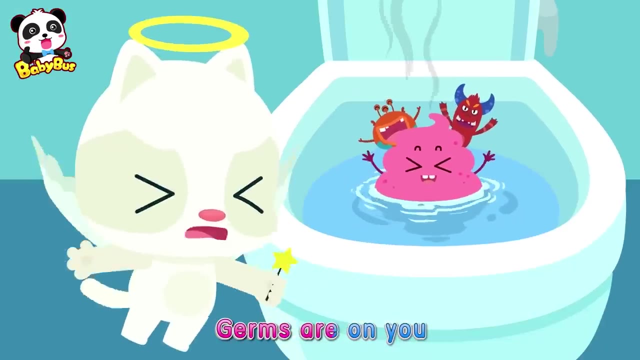 Hurry, Hurry. Should I wash my hands? No, Should I flush it away? No, Let's go out right now. Go, Let's go watch the cartoon. Germs are on you. Germs are on you. Germs are on you. 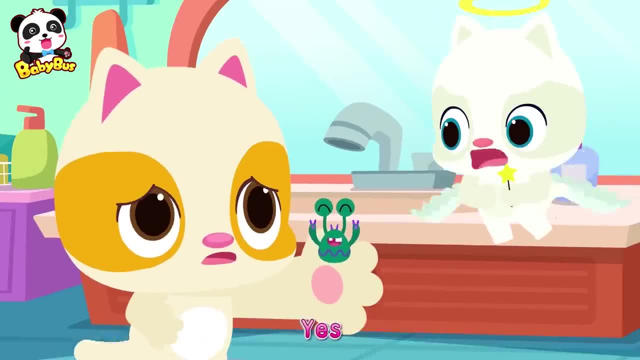 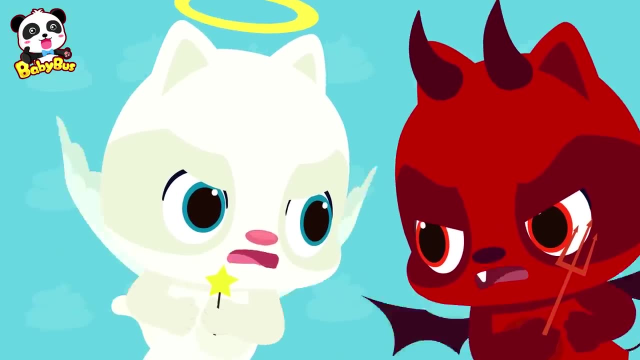 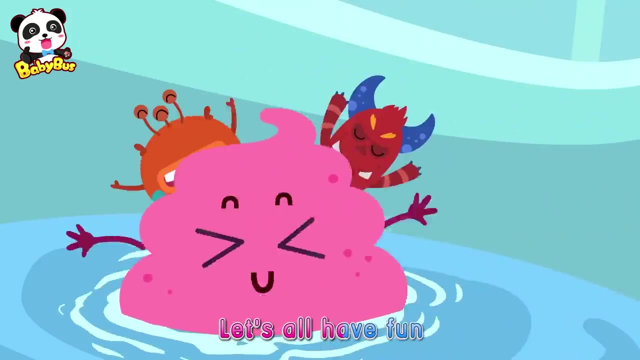 Wait, Wait. Should I wash my hands? Yes, Should I flush it away? Yes, Watch out for the germs. Watch out, They're so noisy, Let's all have fun. Let's all have fun. Let's all have fun. 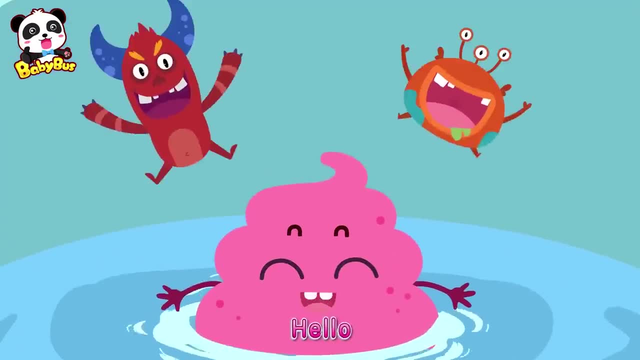 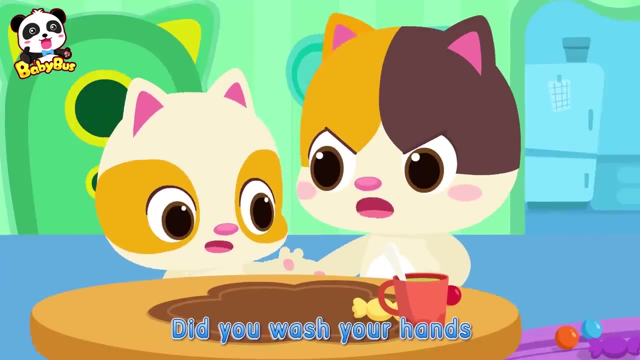 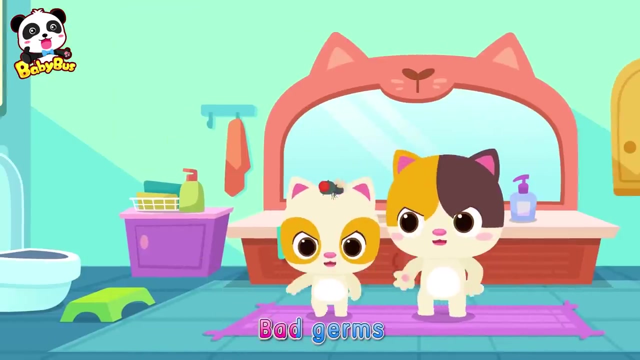 Hooray, Hooray, Germs are back again. They're having fun. Let's all have some fun. Come on, Did you wash your hands? No, There are germs. Go away, bad germs. Go away, bad germs. Go away, bad germs. 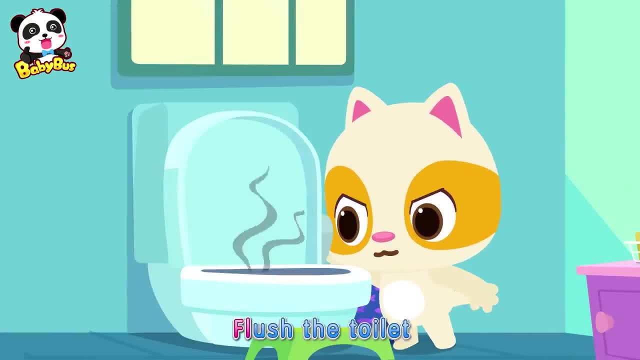 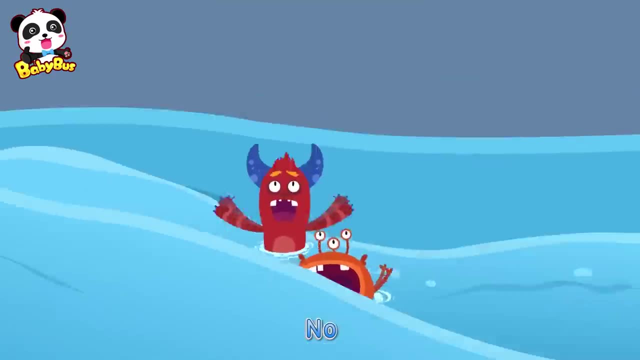 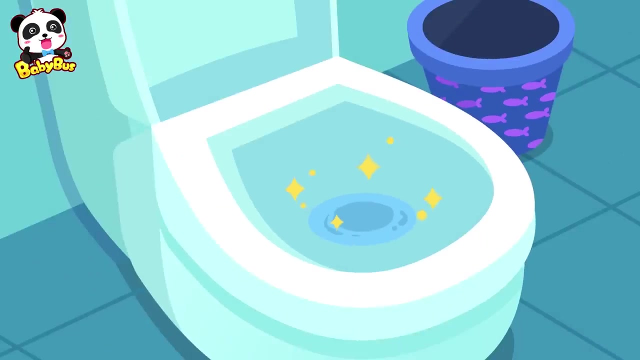 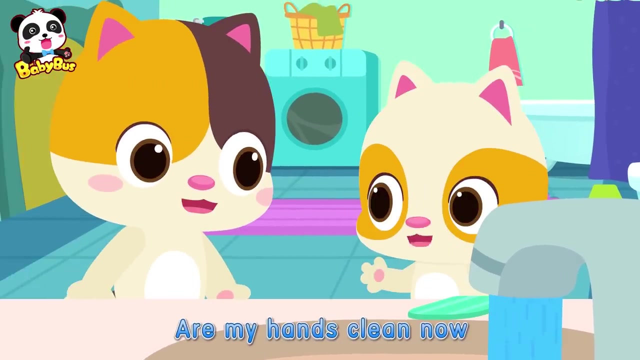 Go away. Push the lever, Okay. Splash the toilet, Okay. Bye-bye, all you germs. Oh, no, No, I don't want to leave. Bye-bye, Help, Do you want my hands clean now? 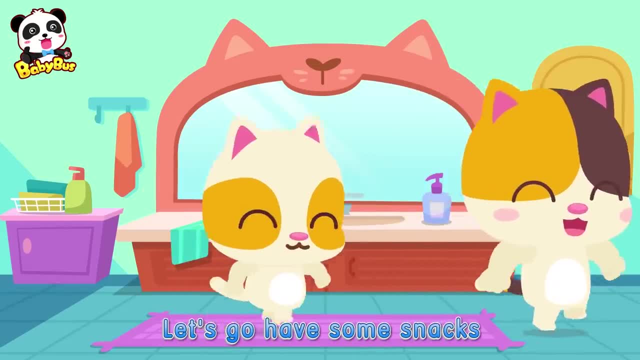 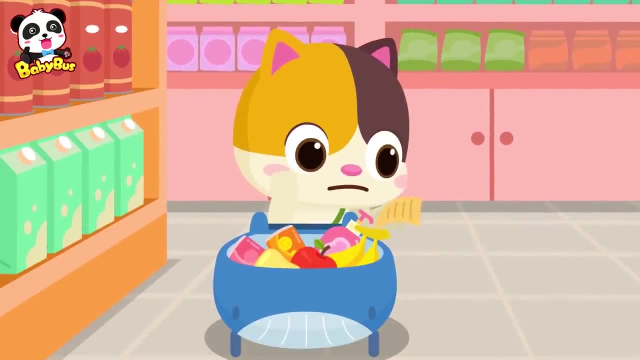 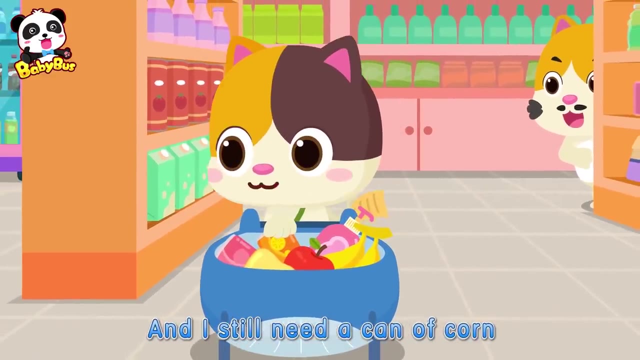 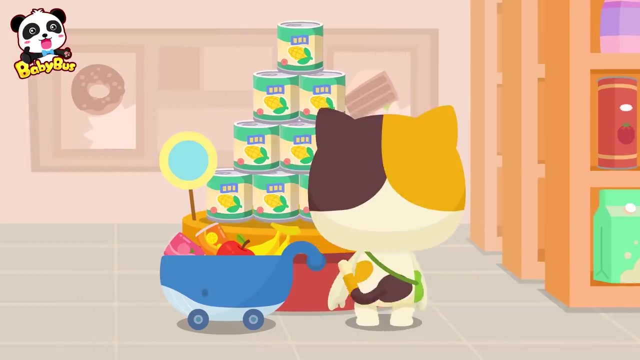 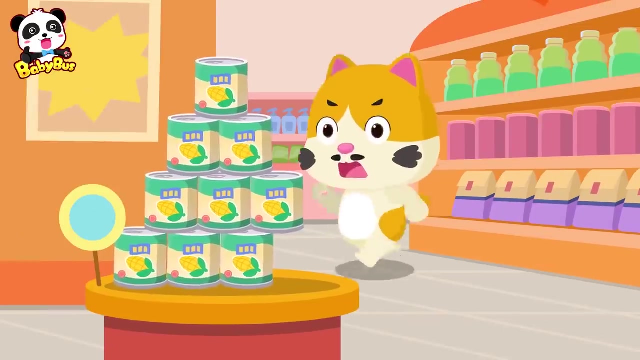 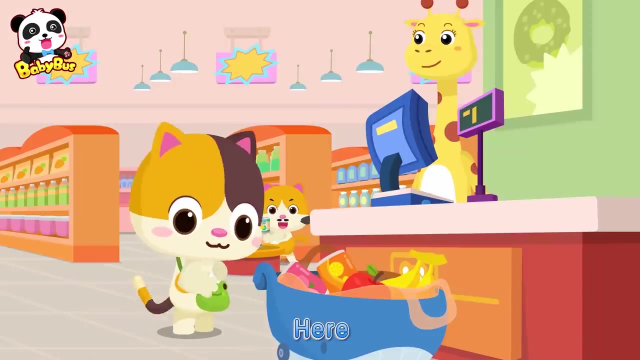 Yes, Let's go have some snacks, And I still need a can of corn, Huh, Okay, Okay, That's it. Oh, Here, Have a nice day. I'm a good girl. I'm buying things for my mom all by myself. 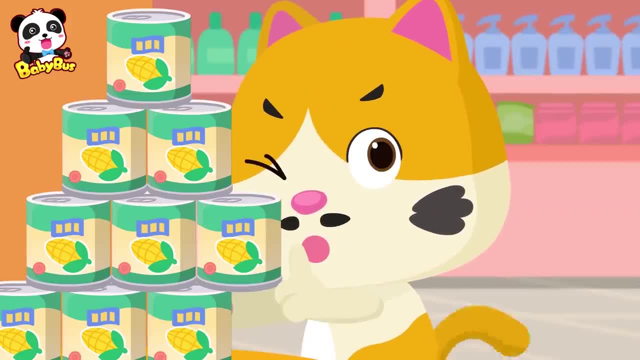 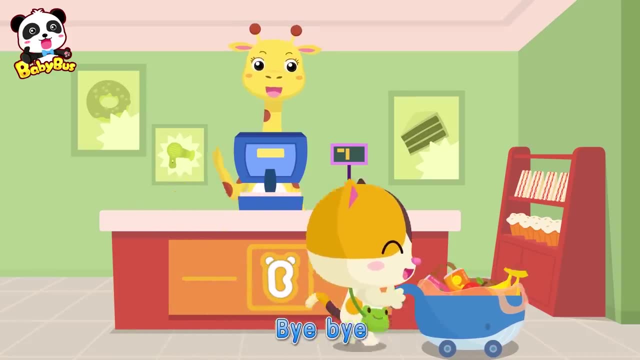 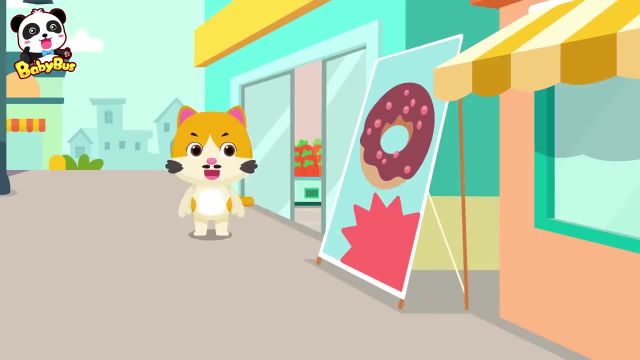 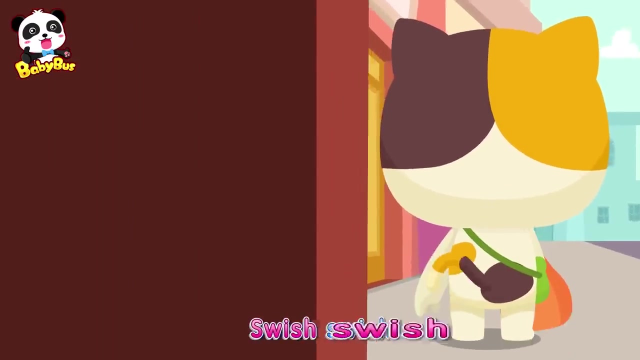 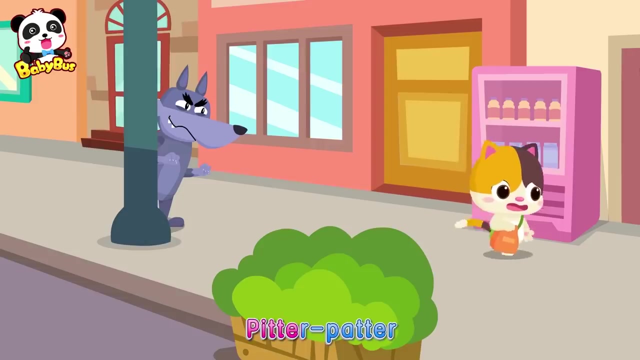 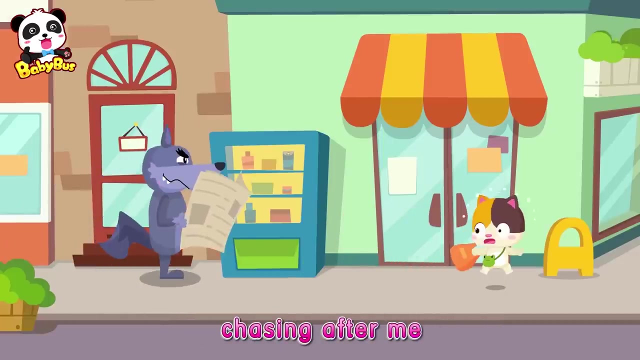 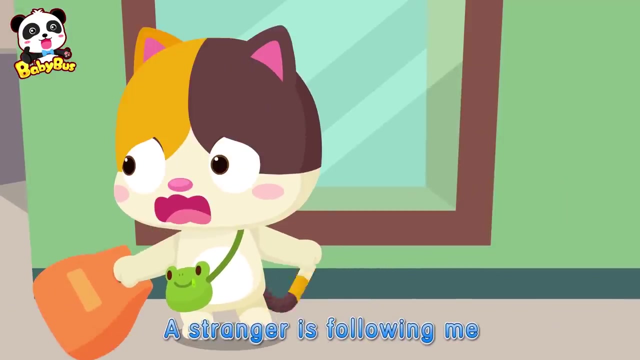 Very good. Bye-bye, Bye-bye, Pitter-patter, swish-swish. I hear someone's footsteps chasing after me. I run, run away from him, But he keeps on coming. Strangers, stay away from me. A stranger is following me. 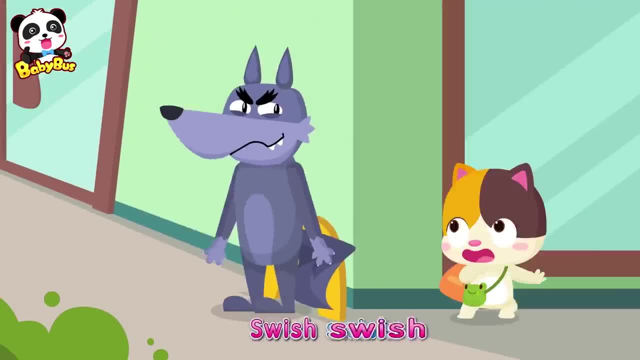 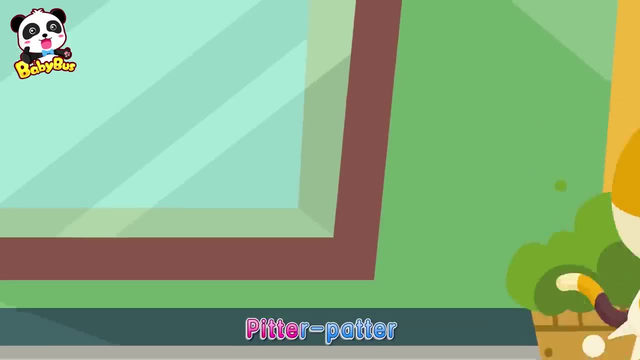 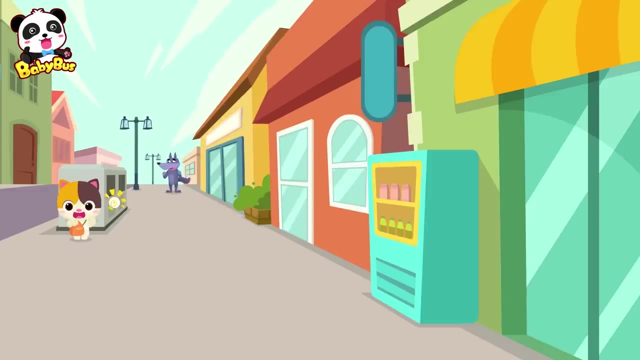 What should I do? Swish swish- swish-swish Pitter-patter run away- Pitter-patter- swish-swish Pitter-patter- swish-swish Pitter-patter- swish-swish. I hear someone's footsteps chasing after me. 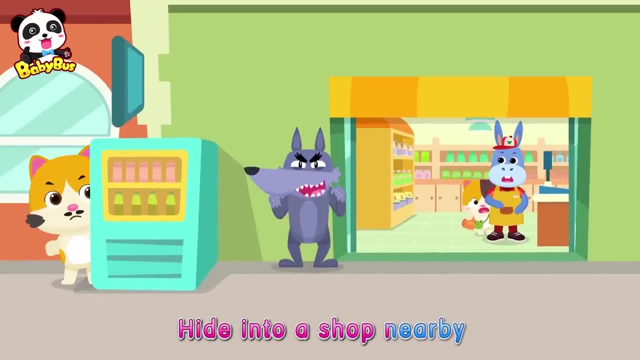 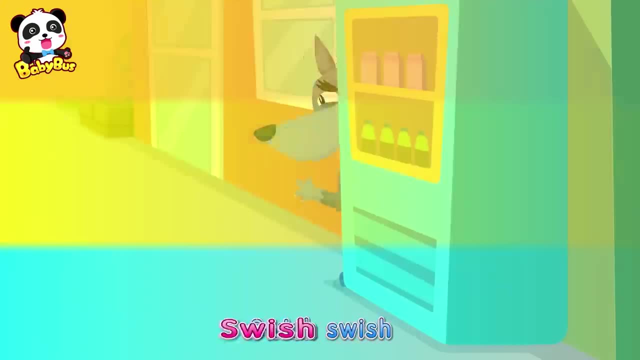 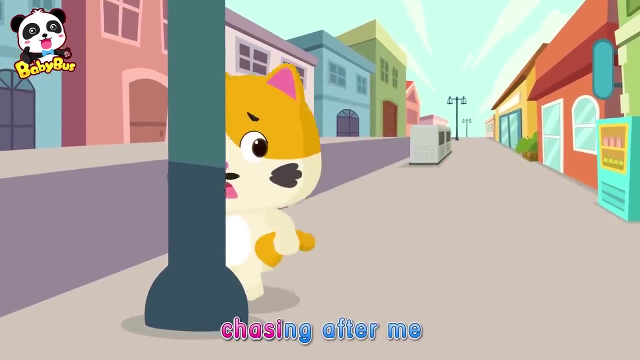 Hurry, hurry, running fast. Hide into a shop nearby. I ask for help. I think it's safe. I can go now. Swish swish, swish-swish, Swish swish. he's back. I hear someone's footsteps chasing after me. 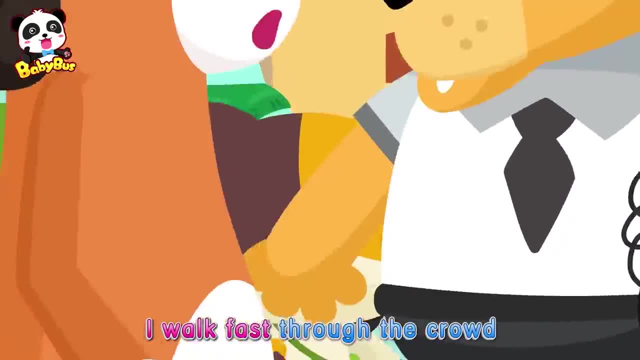 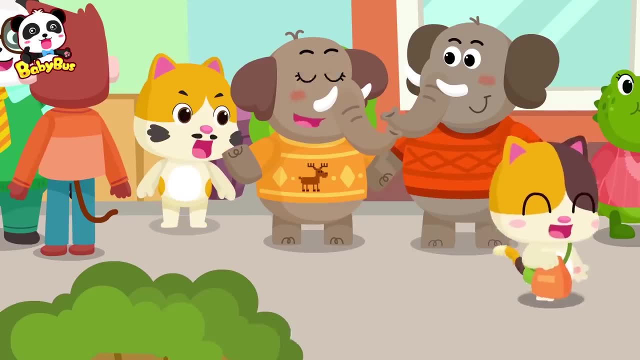 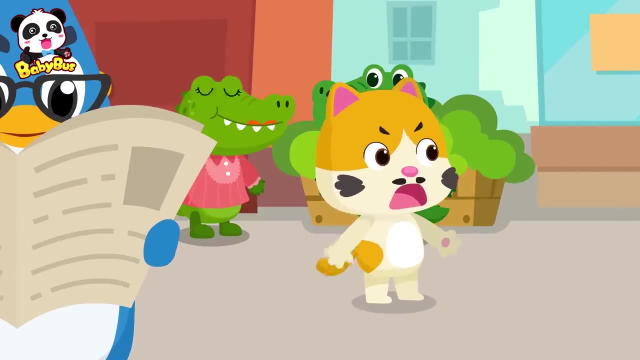 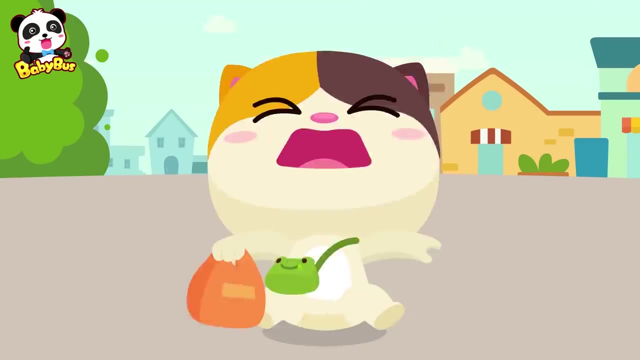 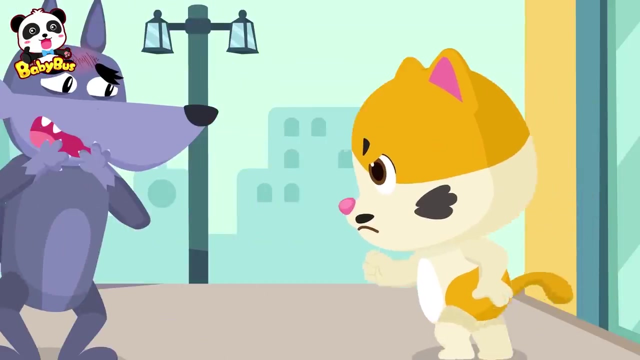 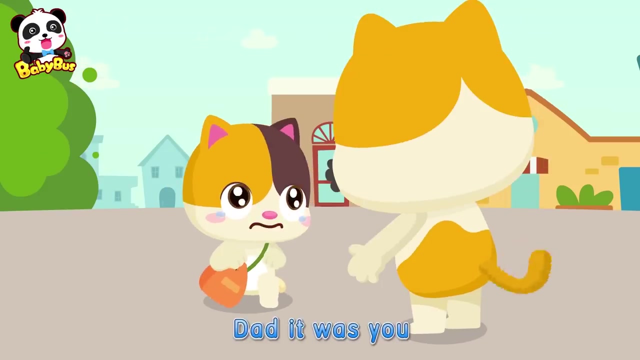 Trying to stay calm. I walk fast through the crowd. The stranger is gone. Phew, Now I can go home. Pitter-patter, pitter-patter, Pitter-patter, let's go home. Oh-oh, Daddy, it was you, Mimi, you're so brave. 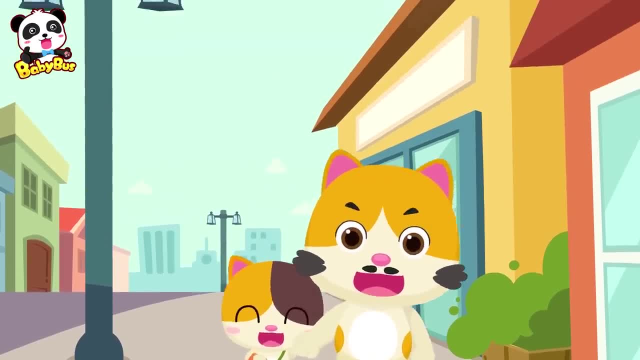 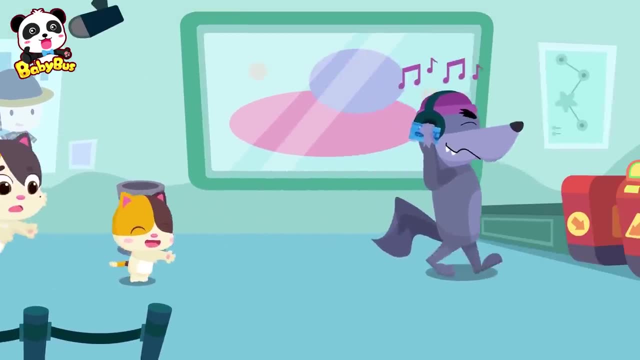 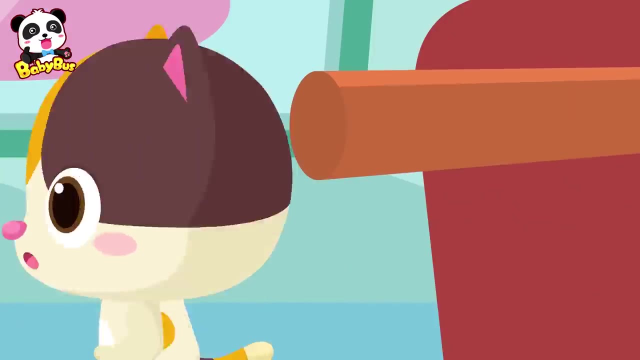 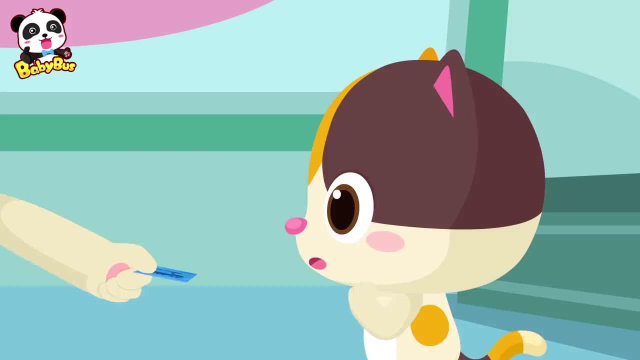 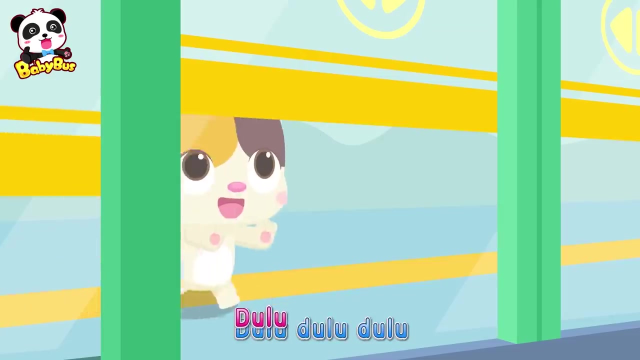 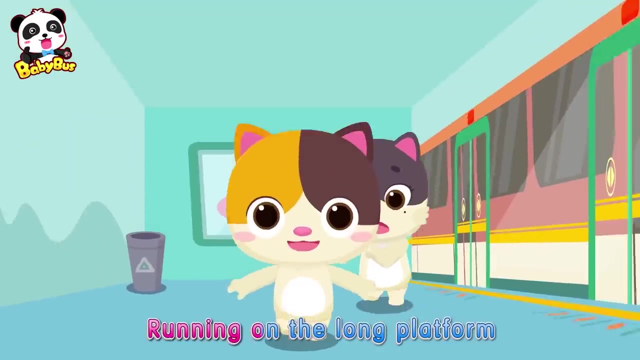 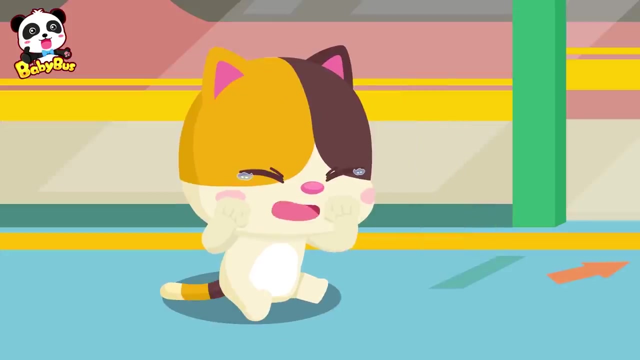 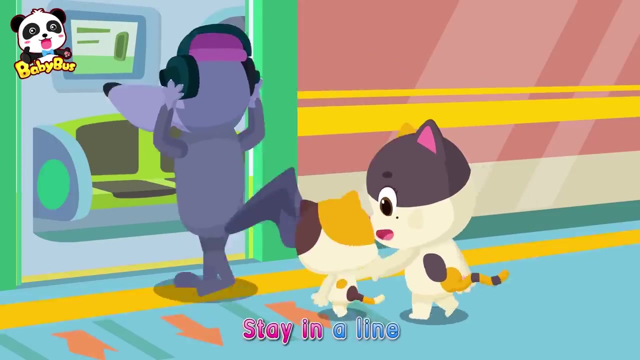 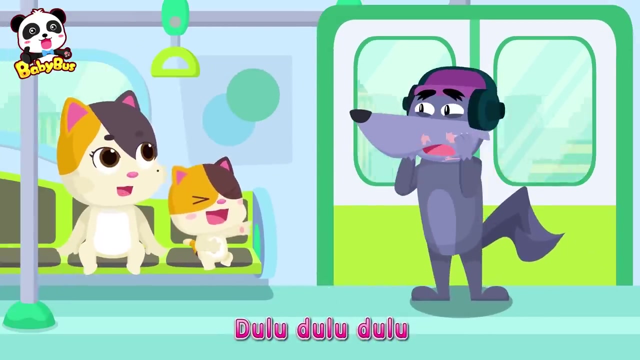 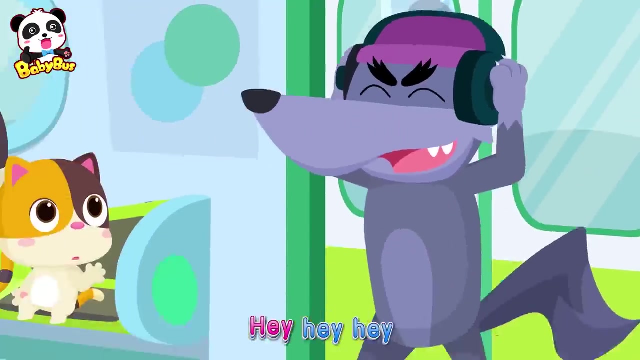 Let's go home together, together, because you didn't use your ticket. when you get on the train, stay behind the safety line. no, no, don't push, stay in a line, watch your step. the train is leaving. go, go, go, leaning on the subway door, hey, hey, hey. 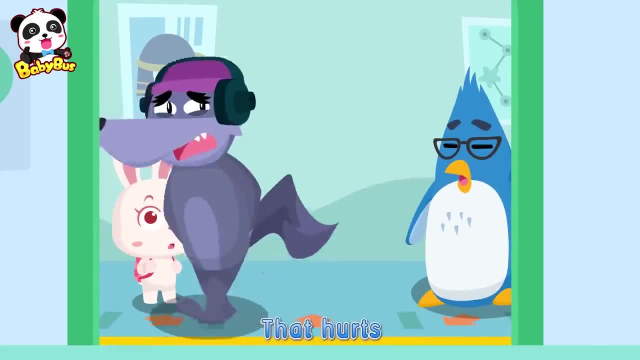 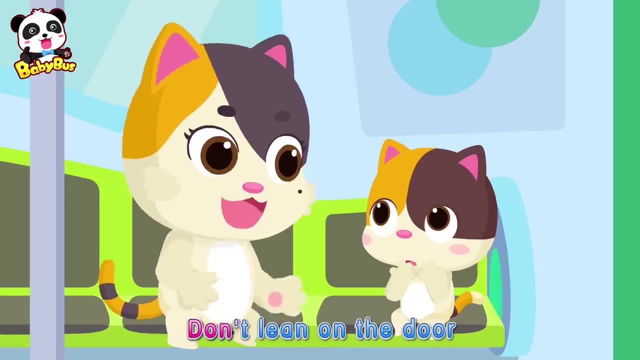 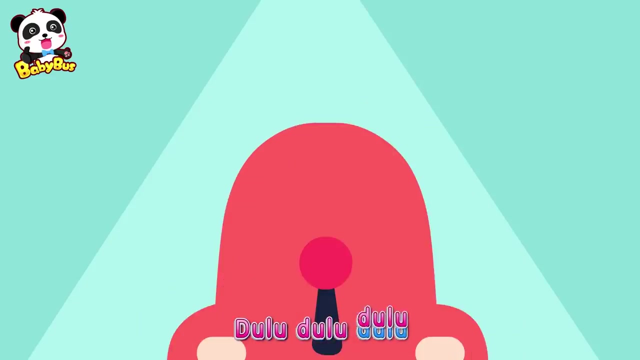 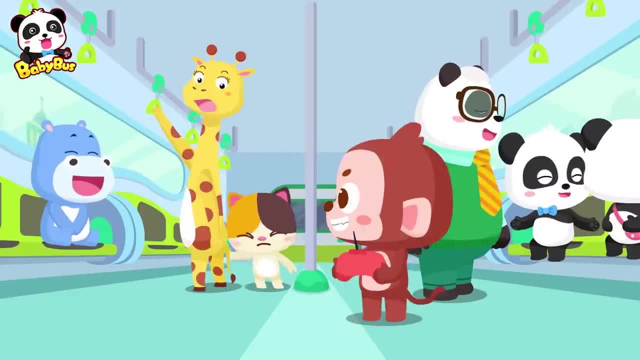 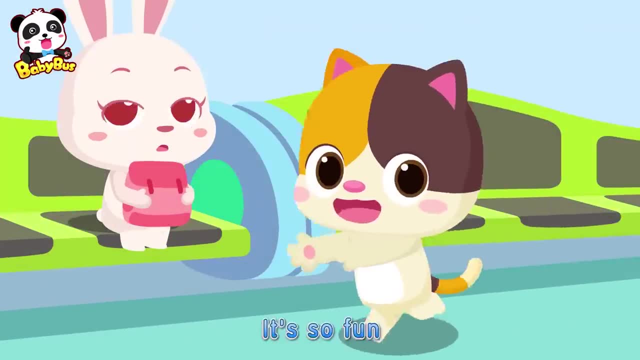 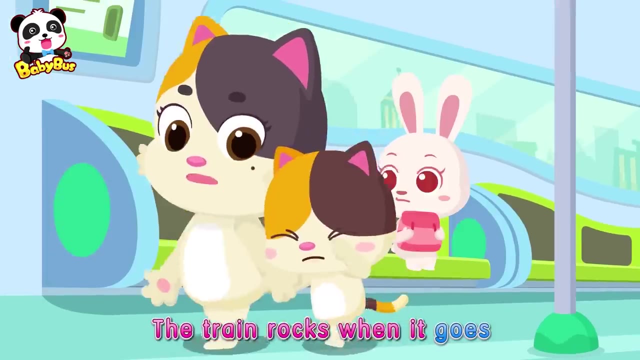 the train is moving, go, go, go. running around here and there shouting out: you can't catch me. golly, golly, golly. it's so fun. be careful when you're on the train. the train rocks when it goes. no, no, don't run in the train. 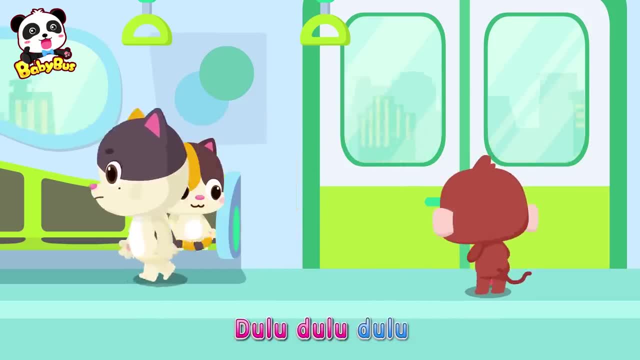 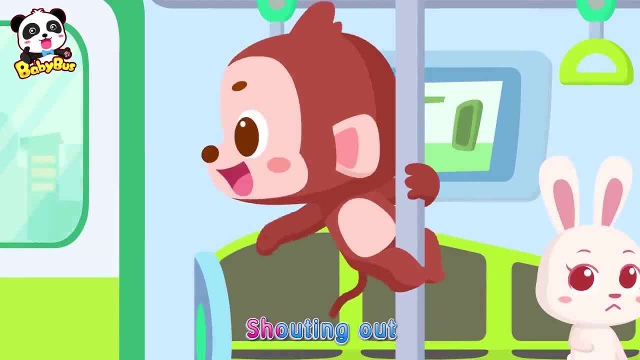 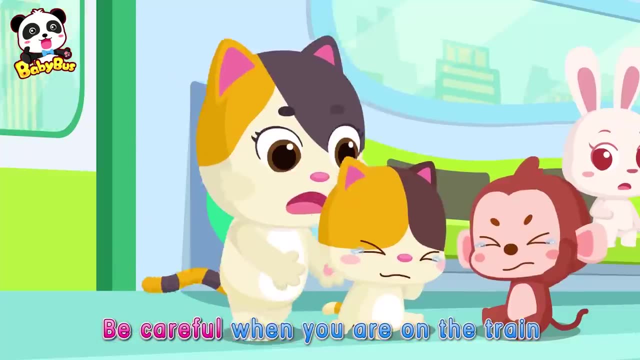 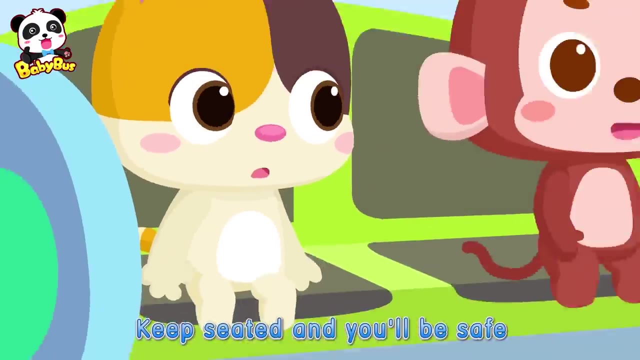 the train is moving. go, go, go, climbing up the pool shouting out: we are so cool, we are so happy and so fun. be careful when you're on the train. the train rocks when it goes. no, no, don't climb up. keep seated and you'll be safe. 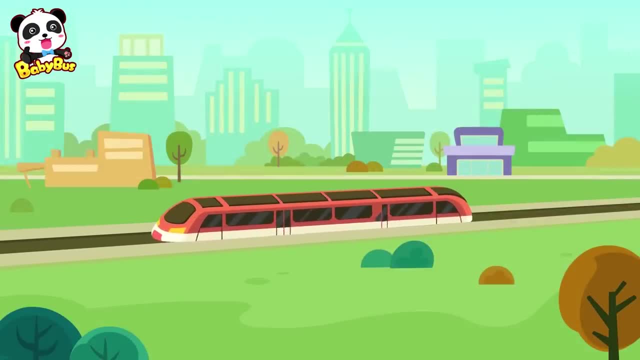 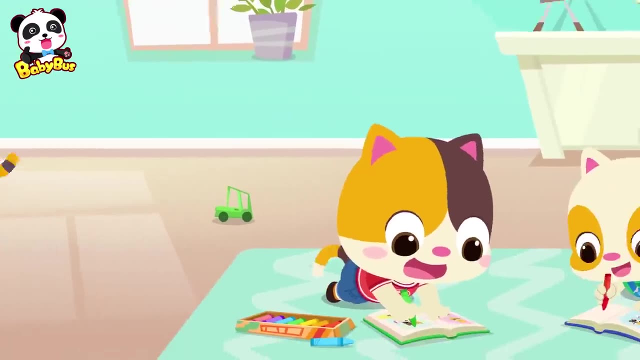 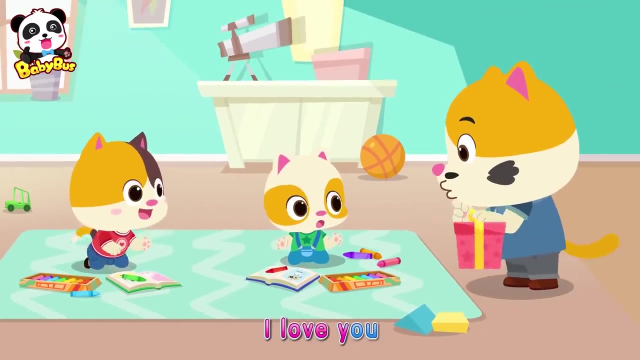 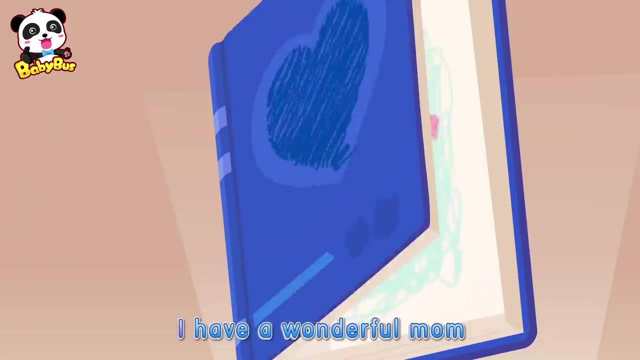 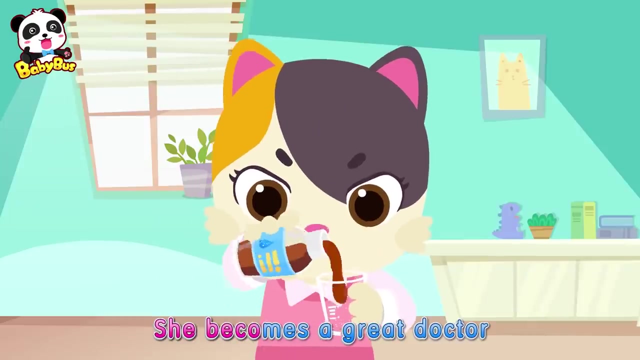 okay, la la, la, la, la la. mommy, I love you. la la, la, la la la. mommy, I love you. la, la, la, la, la la. you're so wonderful. la, la, la, la, la la. I have a wonderful mom. when I feel sick, I need my mom. she becomes a great doctor. 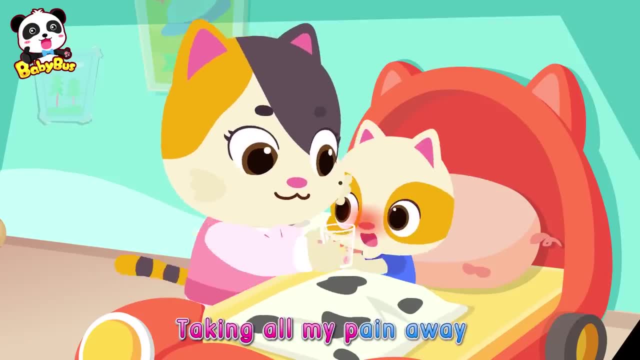 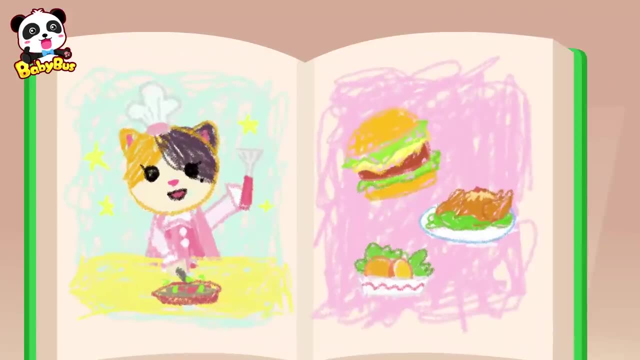 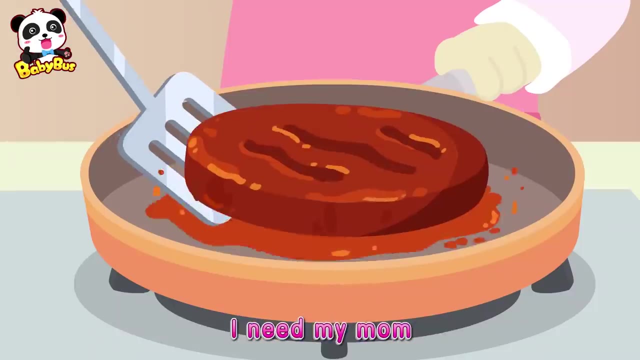 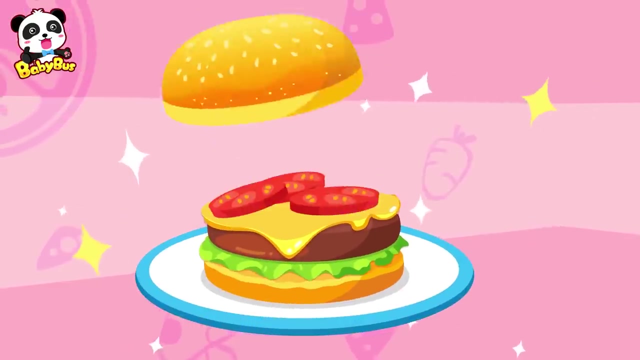 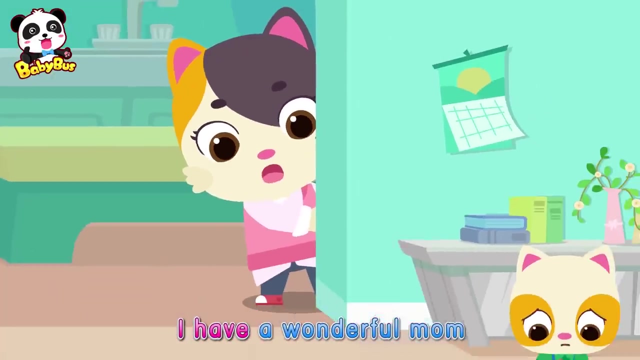 taking all my pain away. I have a wonderful mom. when I feel sick, I have a wonderful mom. When I feel hungry, I need my mom. She becomes a great cook, Making yummy food for me. I have a wonderful mom. When I feel bored, I need my mom. 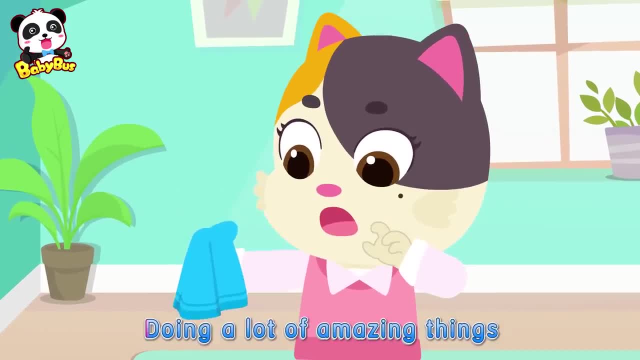 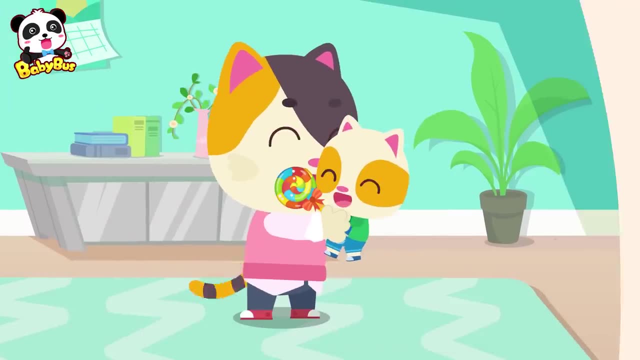 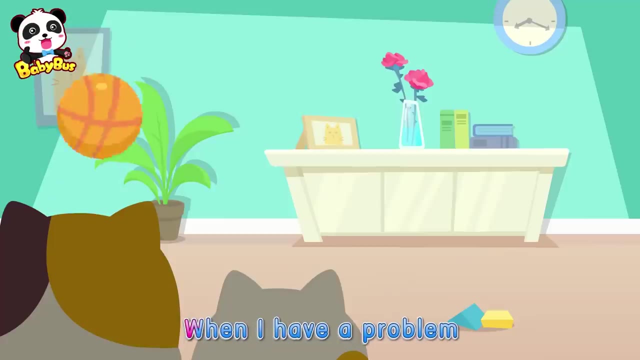 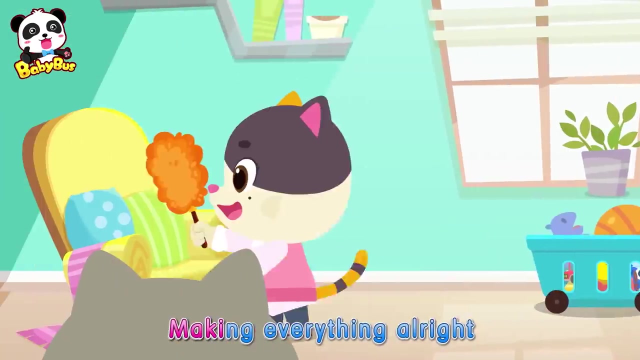 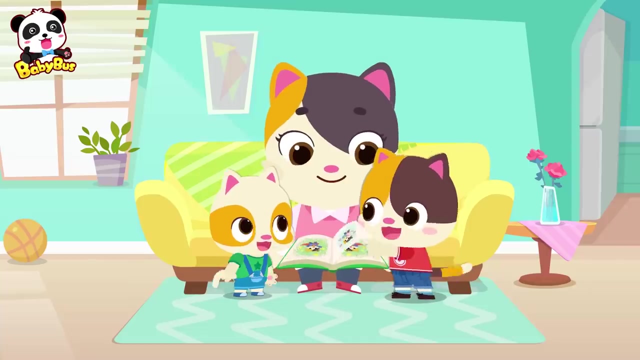 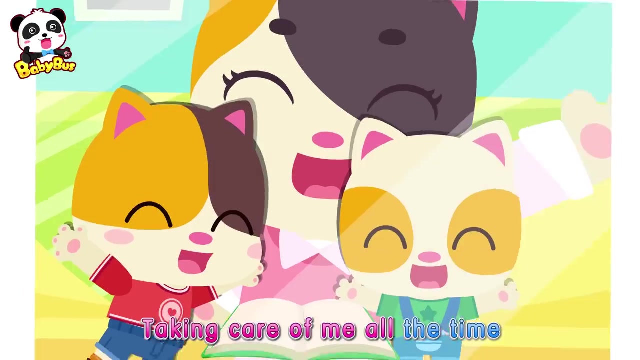 She becomes a great magician, Doing a lot of amazing things. I have a wonderful mom. When I have a problem, I need my mom. She becomes a superhero, Making everything around me. I have a wonderful mom. She takes care of me all the time. You're the best mom in the world. 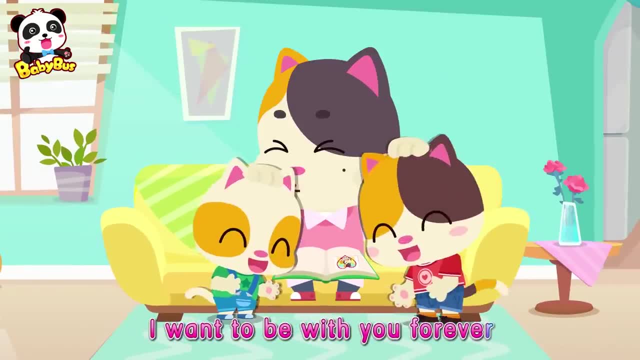 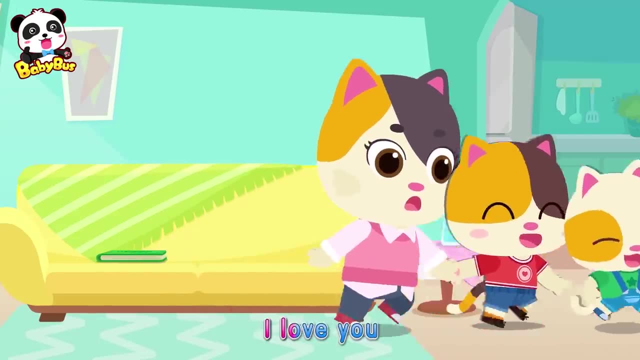 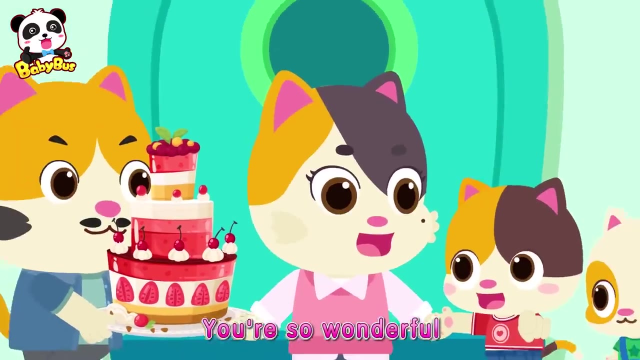 I want to be with you forever. I love you. La la, la, la, la, la, Mommy, I love you. La la, la, la, la, Mommy, I love you. La, la, la, la, la, la. You're so wonderful. La la, la, la, la la. Come here. 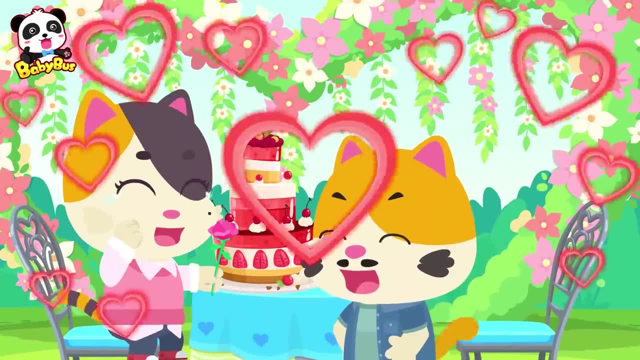 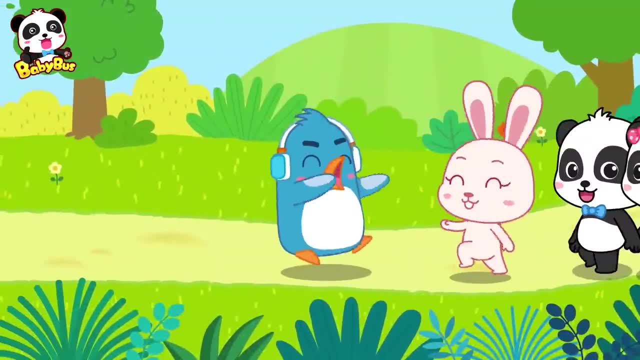 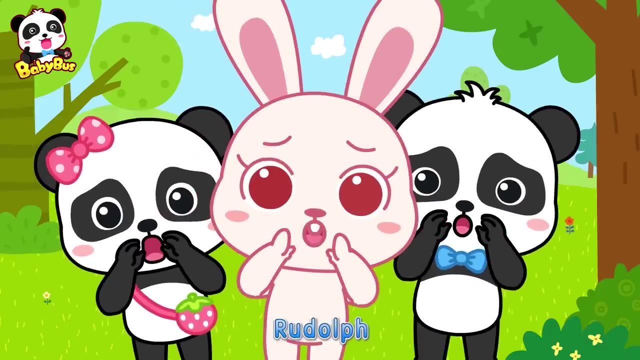 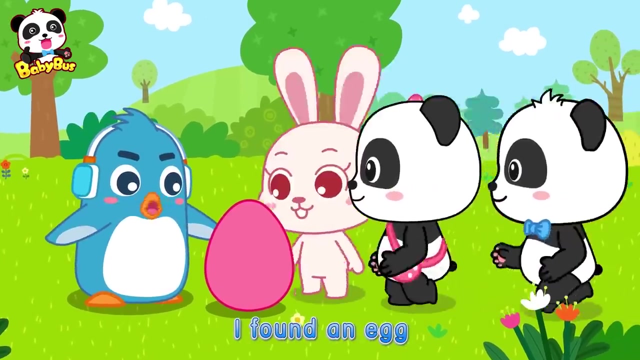 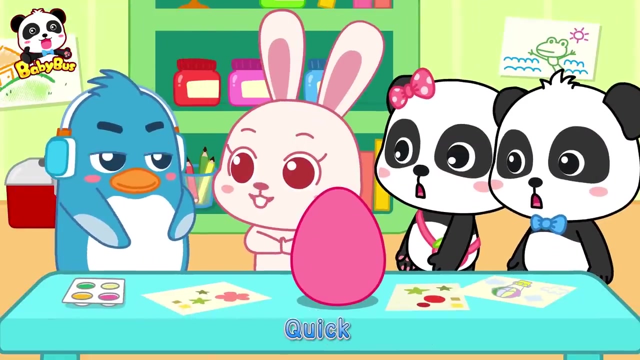 Wow, Oh wow, Oh wow, Wow, Oh yeah, Wow, Rudolph, Ouch, That hurts, Huh. Hey, look at this, I found an egg. Whoa, Is it a surprise egg? Quick, let's open it up. 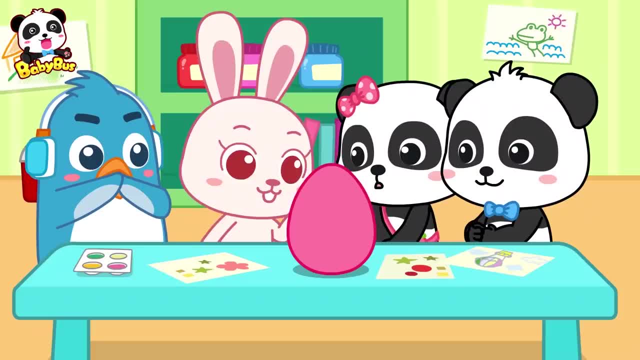 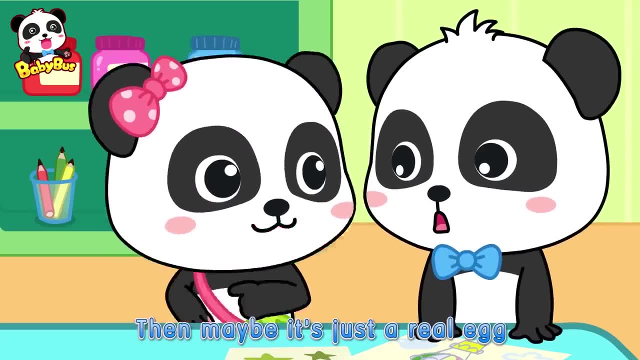 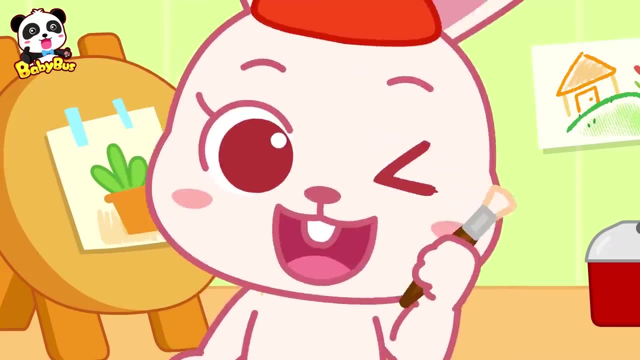 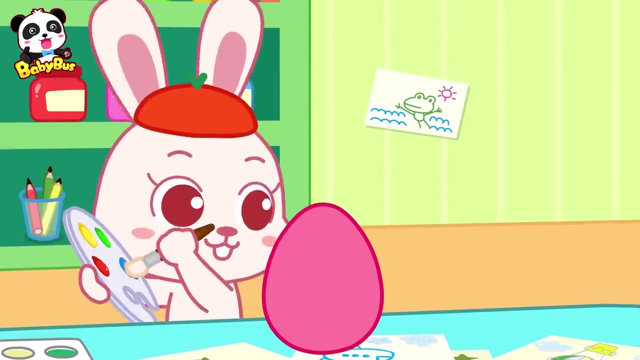 Maybe there are candies and cookies inside. Huh, Look, It's not a surprise egg. Then maybe it's just a real egg, A real egg. How should we take care of it? Let me try: Little egg, little egg. I'll take care of you. 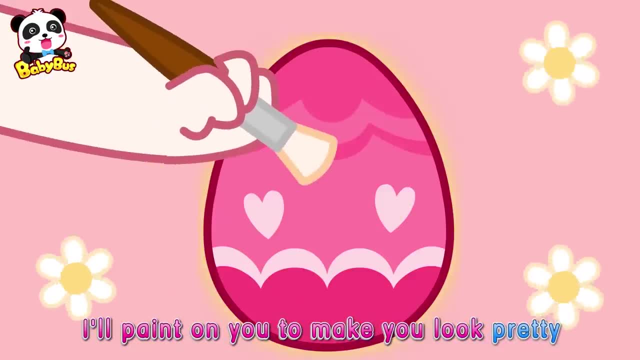 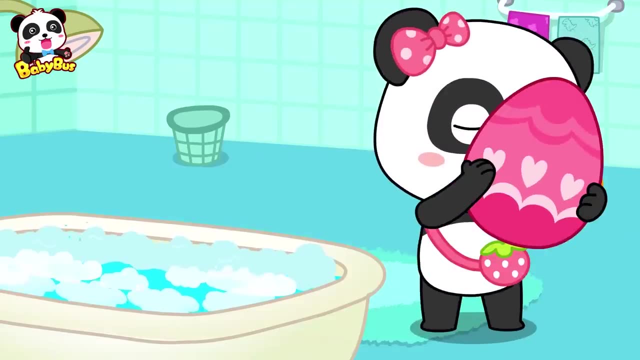 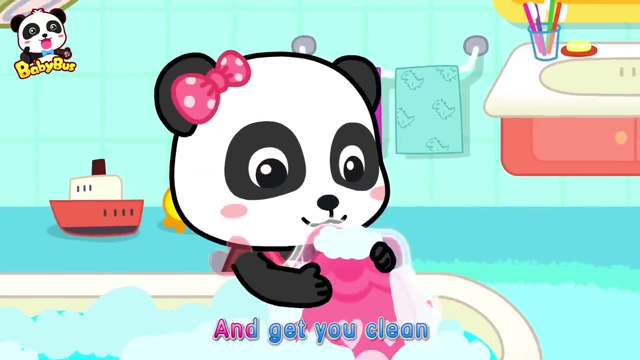 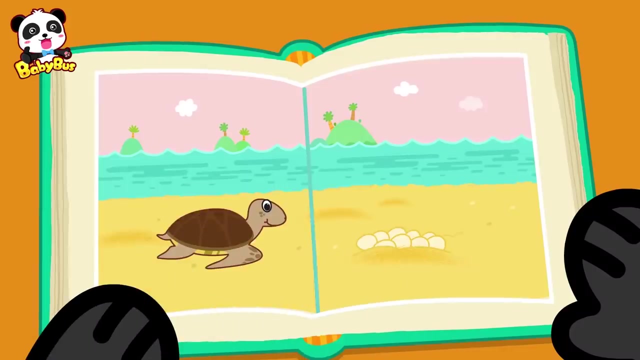 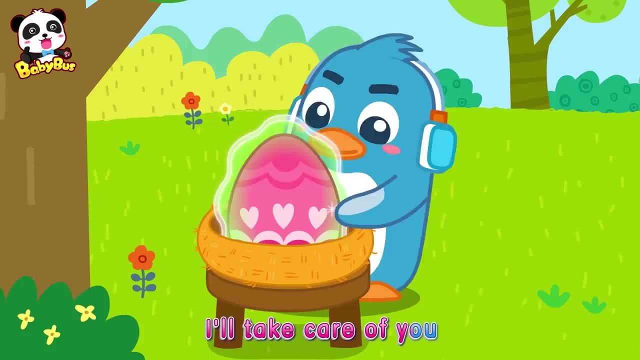 I'll paint on you to make you look pretty. No, that's not right. Little egg, little egg. I'll take care of you. I'll give you a bubble bath and get you clean. Little egg, little egg. I'll take care of you. 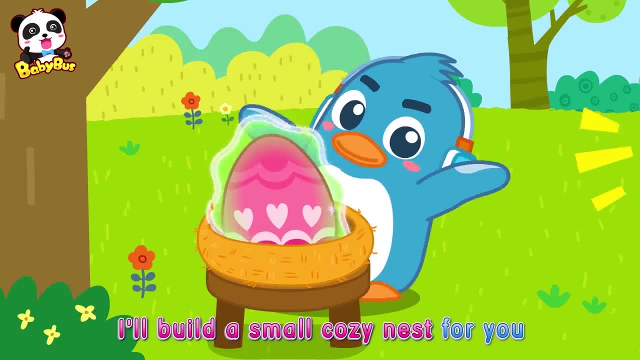 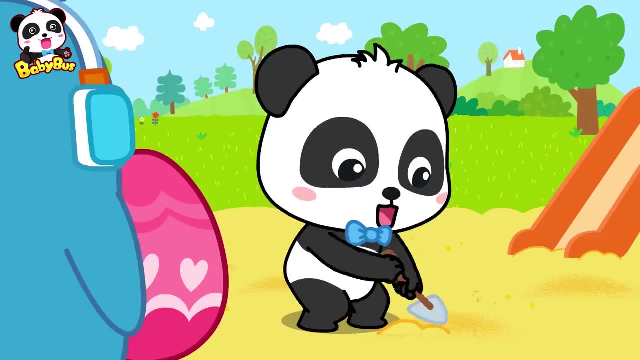 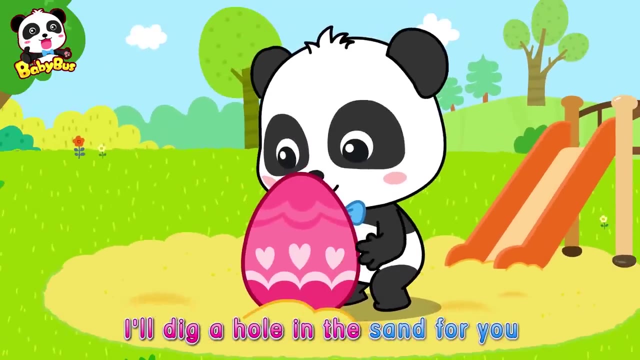 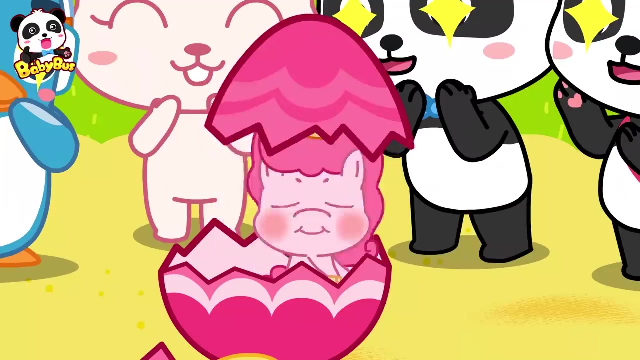 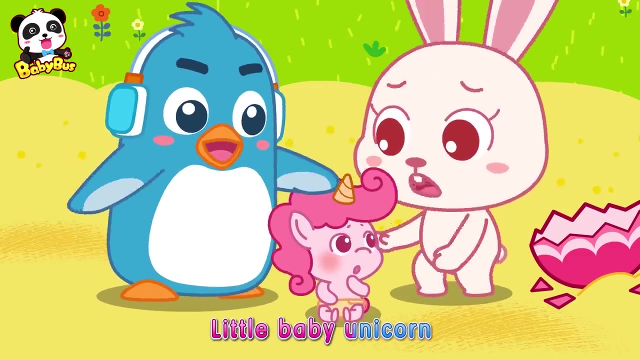 I'll build a small cozy nest for you. No, that's not right. Little egg, little egg. I'll take care of you. I'll dig a hole in the sand for you. Wow, It's a unicorn. She seems hungry. Little baby unicorn, I'll take care of you. 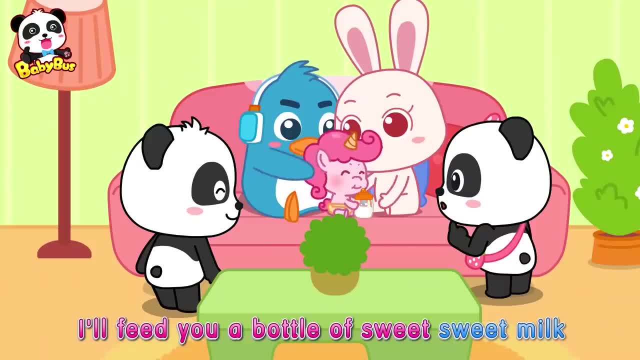 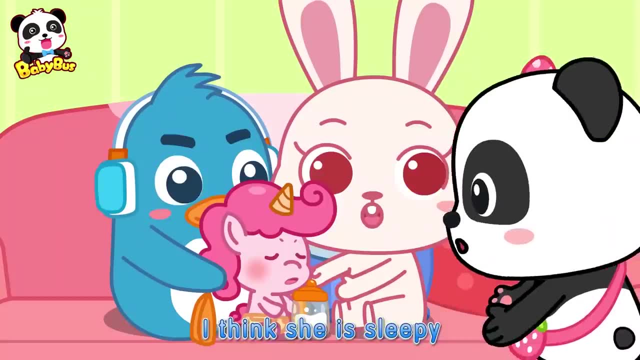 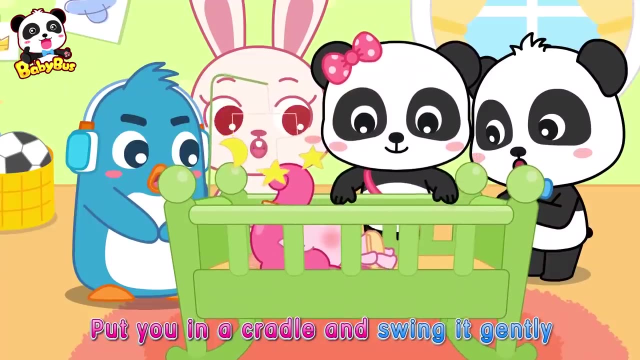 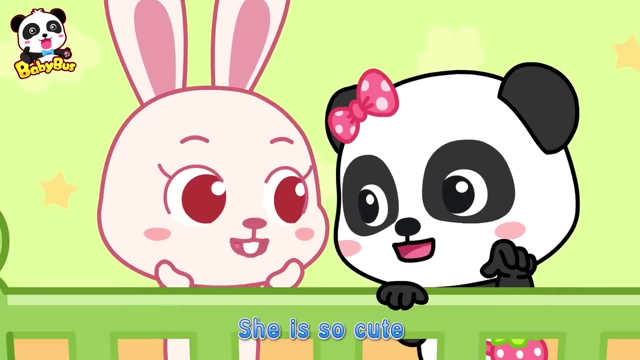 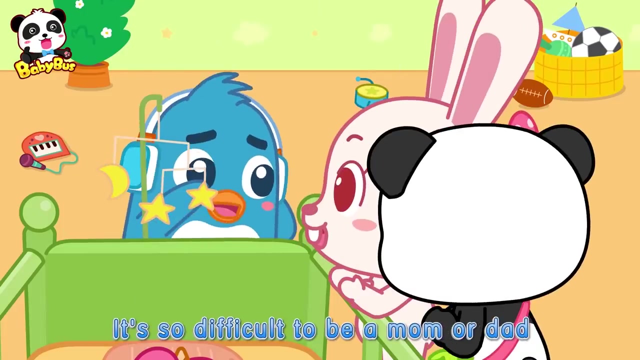 I'll feed you a bottle of sweet, sweet milk. Wow, I think she's sleepy Little baby unicorn. I'll take care of you, Put you in a cradle and swing it gently. She is so cute. We became parents. It's so difficult to be a mom or a dad. 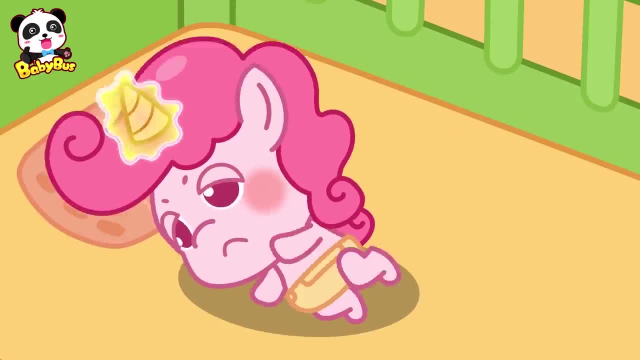 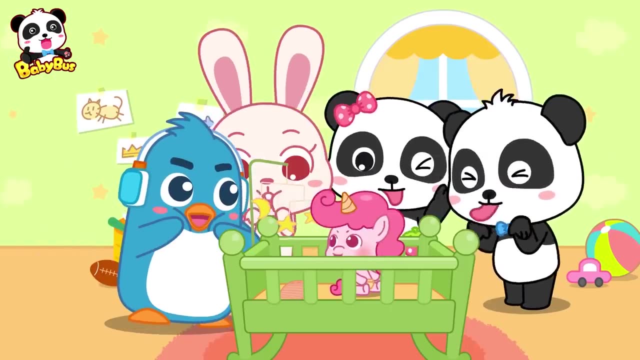 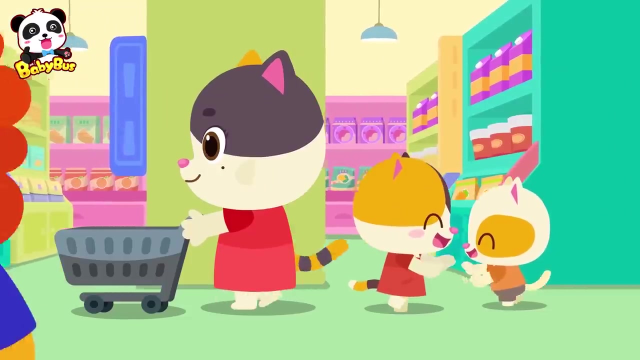 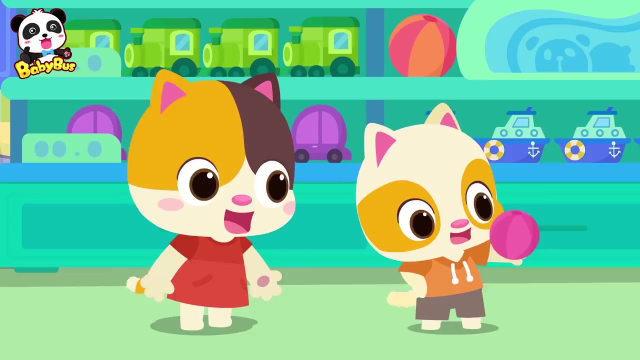 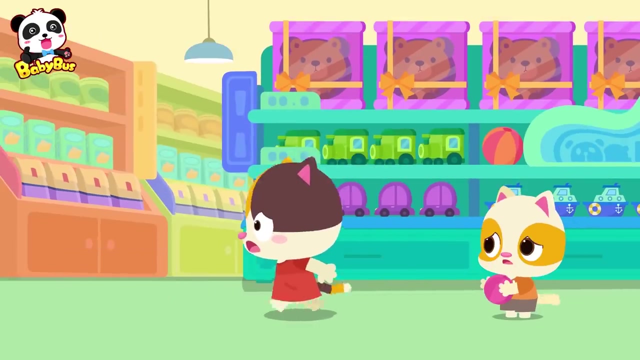 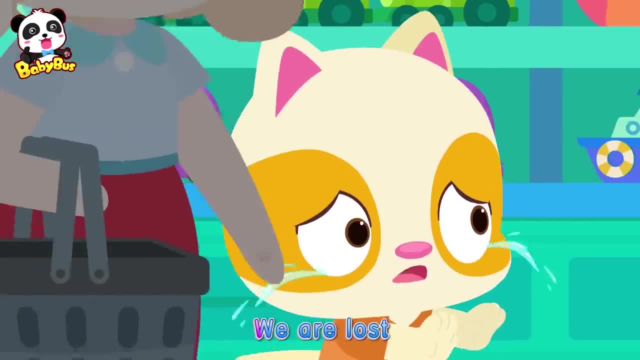 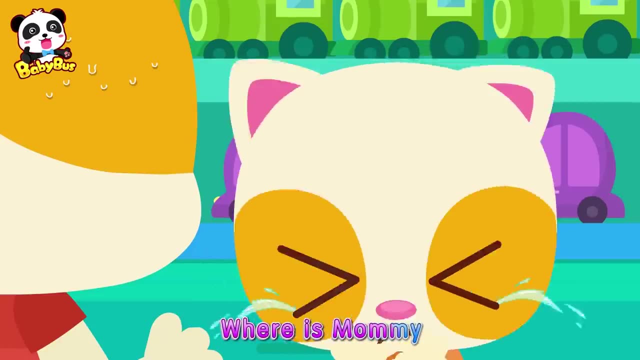 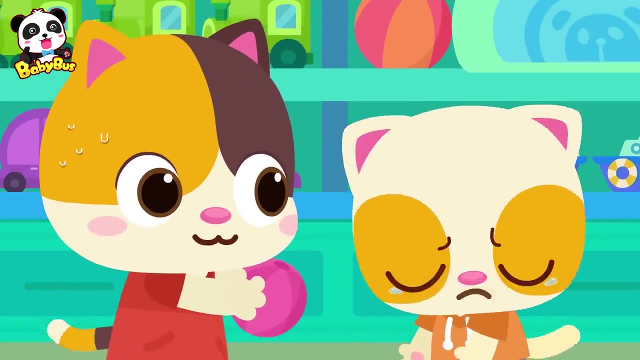 We're lost, Oh, we are lost, Oh, we are lost. I'm so scared. Oh no, Oh no. Where is mommy? Don't worry, Listen to me, Let's wait for mommy here, Don't worry. 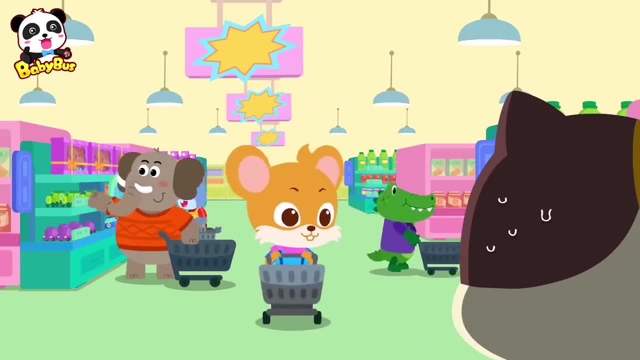 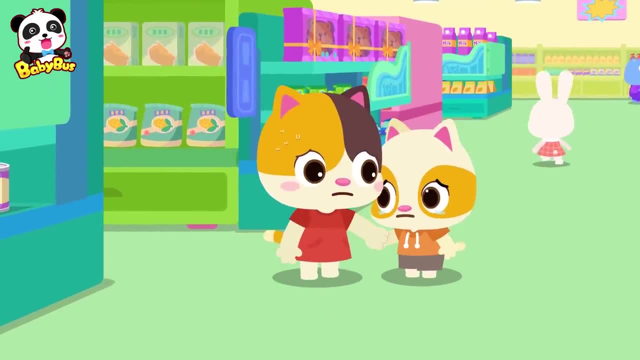 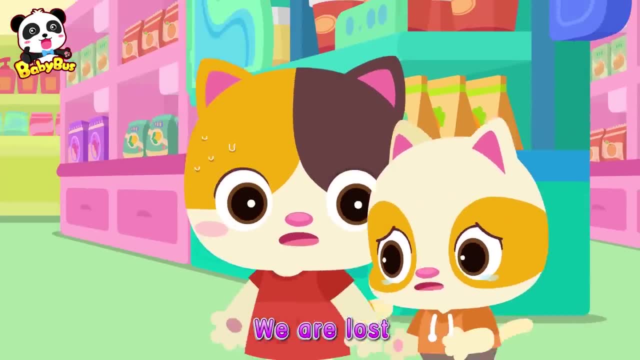 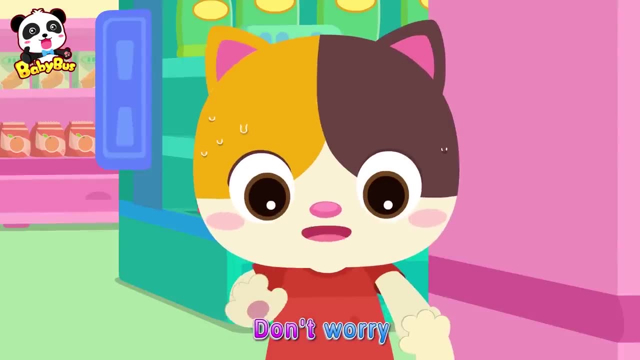 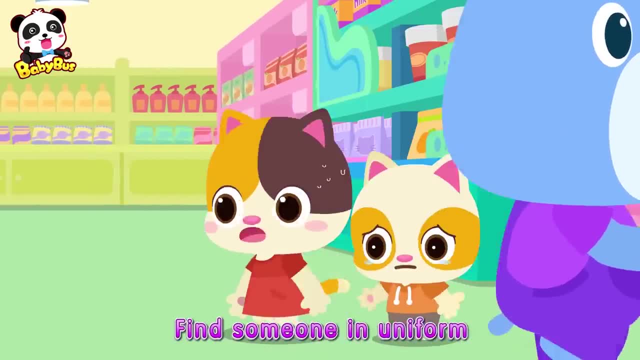 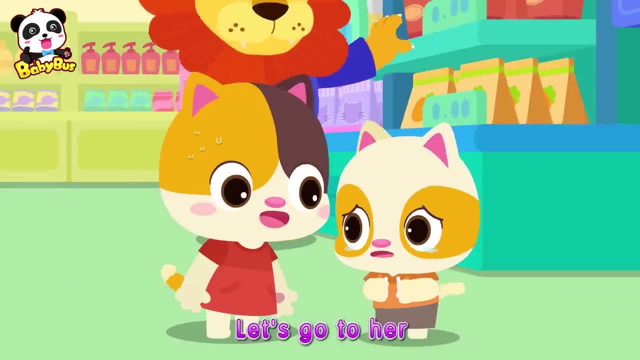 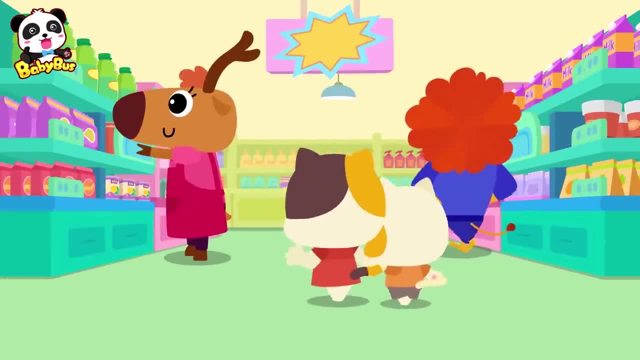 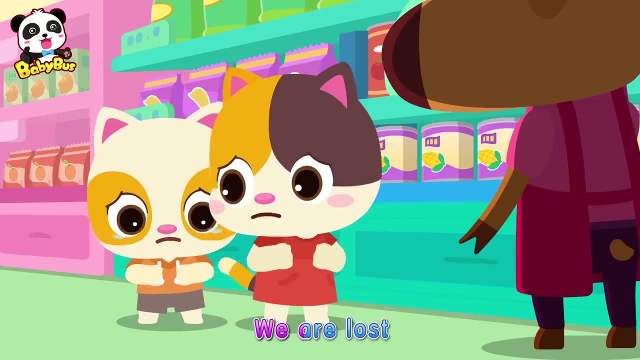 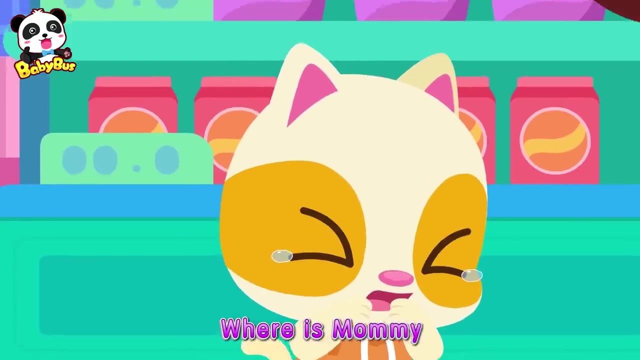 Mommy is back. Ask her for help. Kids, how can I help you? All we are lost. all we are lost. Please help find our mom. Oh no, Oh no. Where is mommy? Little kids, don't be scared. 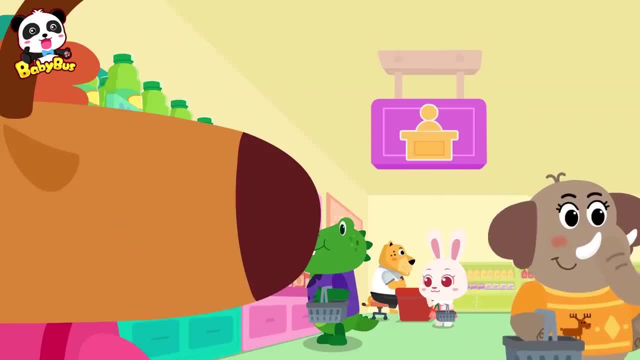 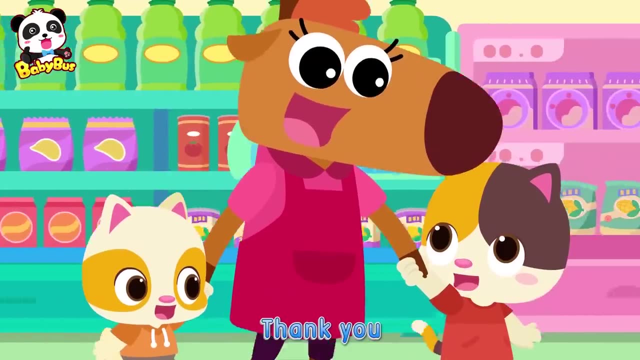 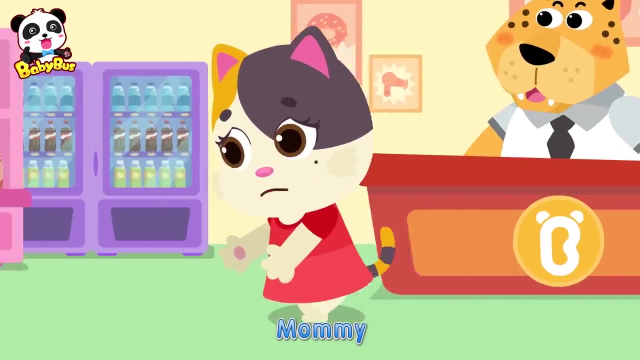 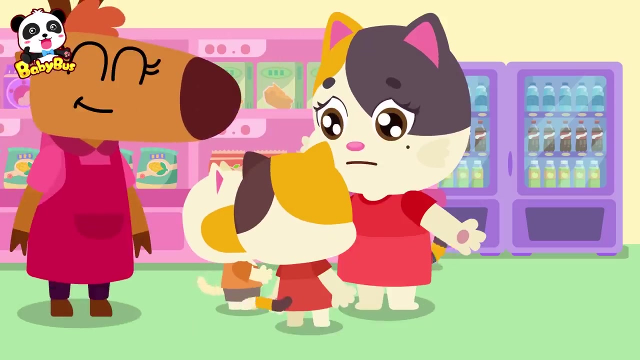 I'll help you find your mom, Don't worry. don't worry, Follow me, little kids. Thank you, It's mommy. Mommy, Mommy, Mommy, Timmy, Help, Help, Where have you been? We got lost. 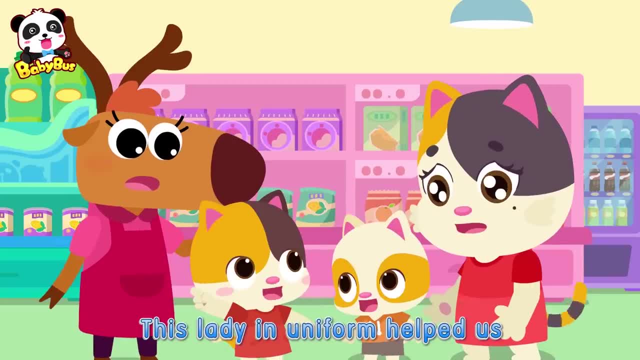 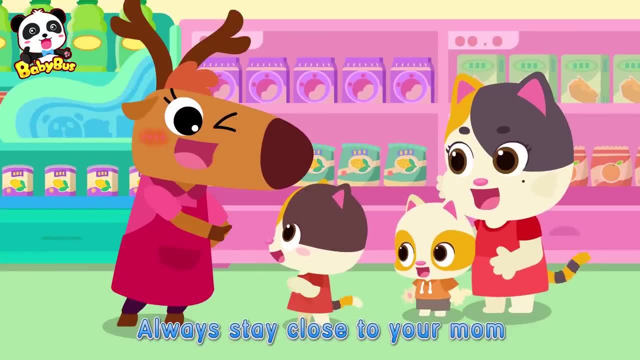 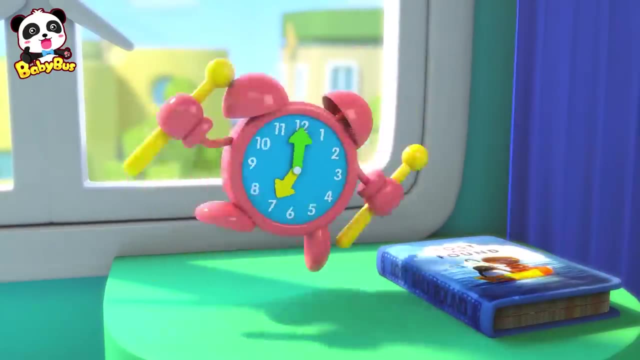 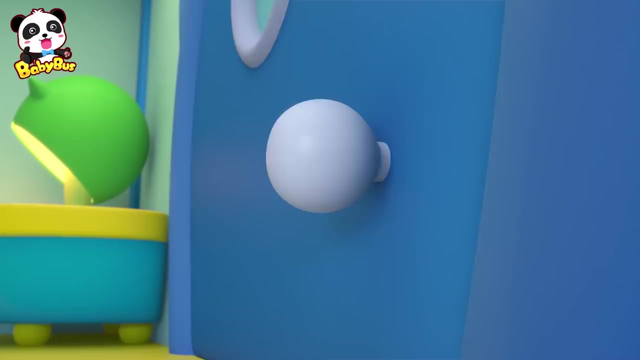 Yes, This lady in uniform helped us. Thank you, You're welcome. Always stay close to your mom. Okay, I am home. I'll be back soon. It's time to go. Let's go. We're going up to the sky with mom. 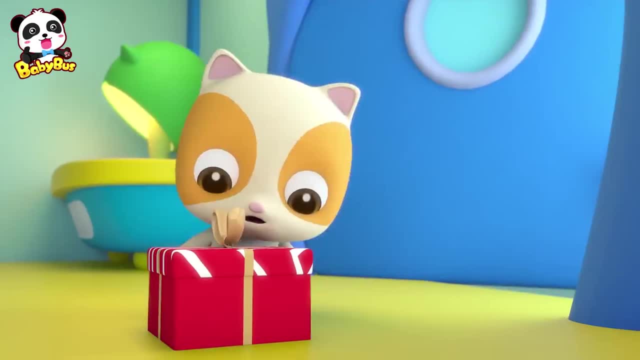 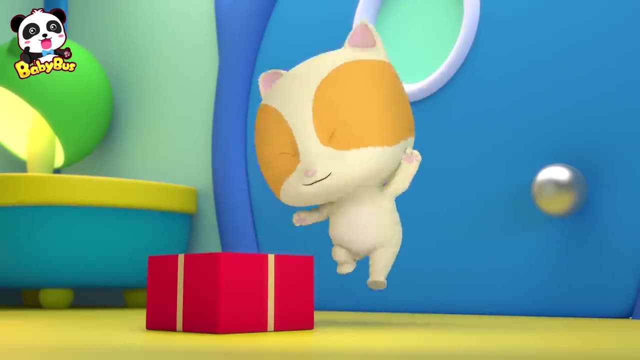 We'll get up on the plane out of the clouds. Okay, Okay, We can't stay up here. Just stay down. No, Stay down. Oh, stop Please. Why is that What I? What's going on? 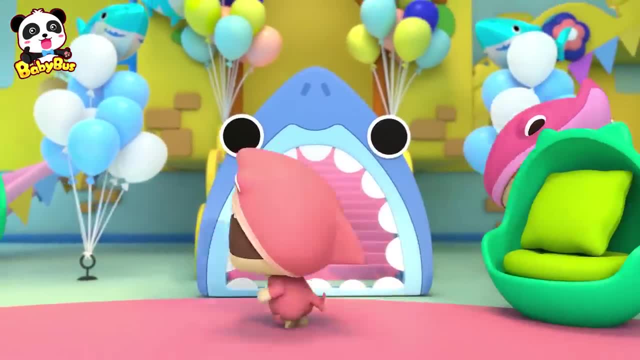 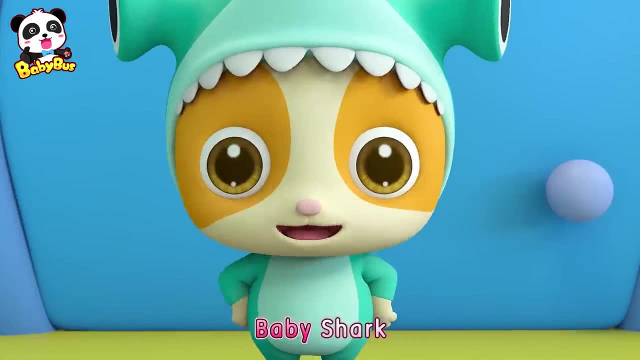 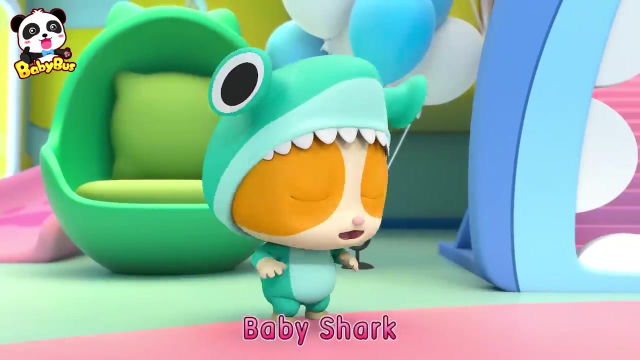 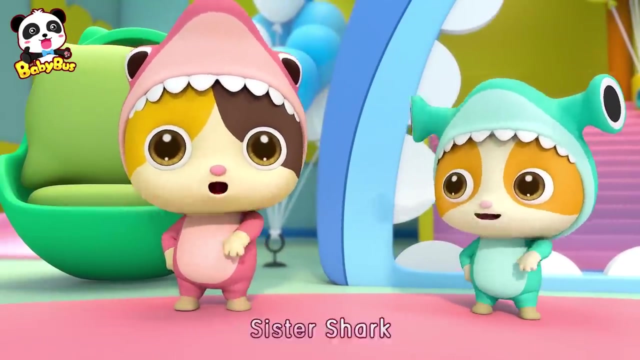 I. I. Baby Shark. do-do-do-do-do Baby Shark. do-do-do-do-do Baby Shark. do-do-do-do-do Baby Shark. Sister Shark. do-do-do-do-do Sister Shark. do-do-do-do-do Sister Shark. do-do-do-do-do Sister Shark. 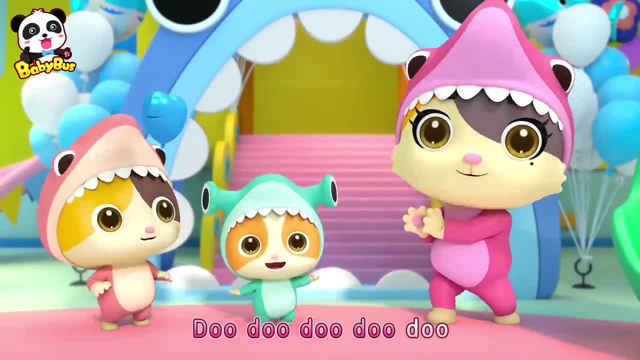 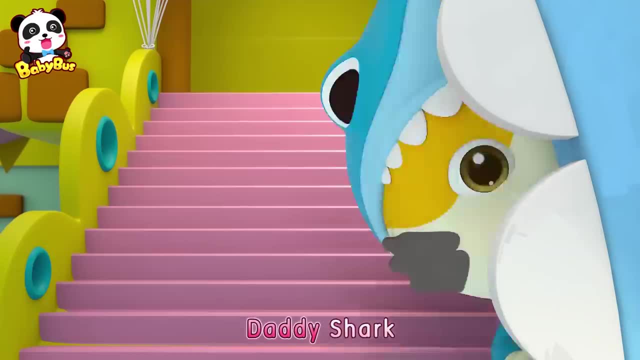 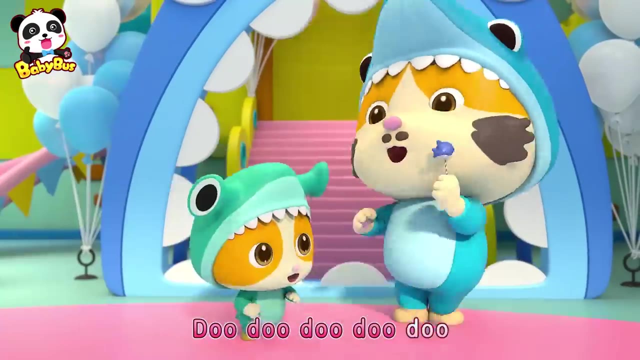 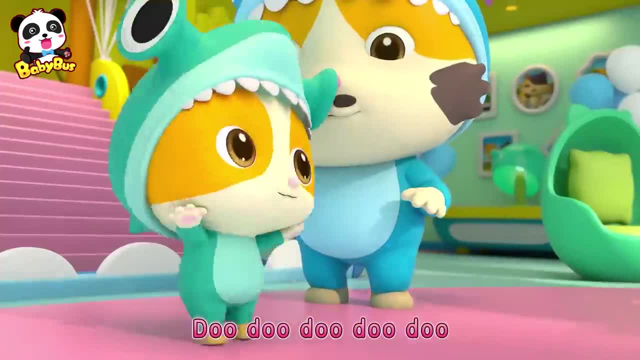 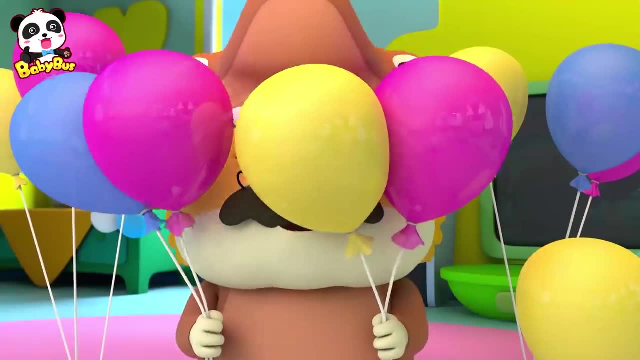 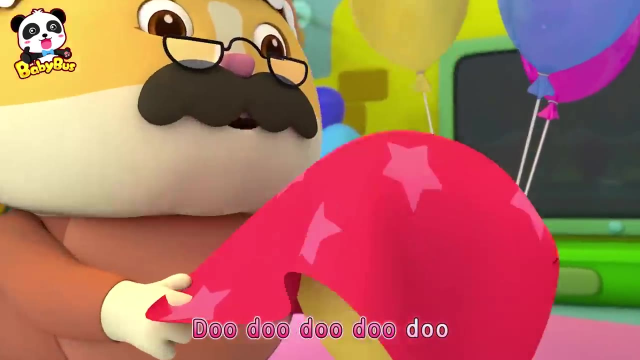 Grandma shark, do-do-do-do-do. Grandma shark, do-do-do-do-do, Grandma shark, do-do-do-do-do, Grandma shark. Grandpa Shark, doo-doo-doo-doo, Grandpa Shark, doo-doo-doo-doo, Grandpa Shark, doo-doo-doo-doo, Grandpa Shark. 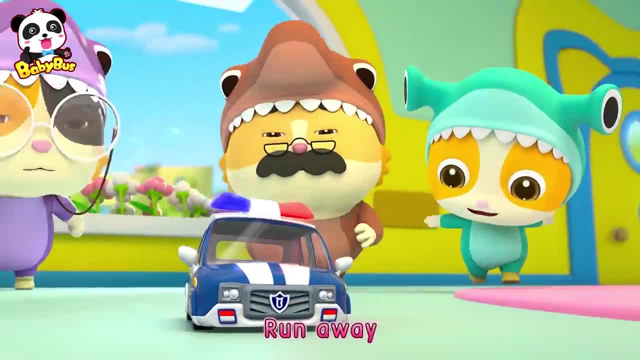 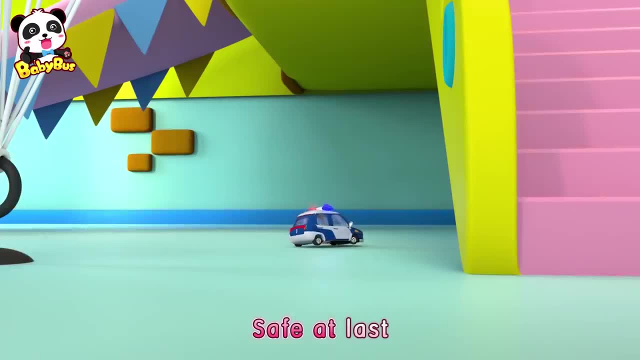 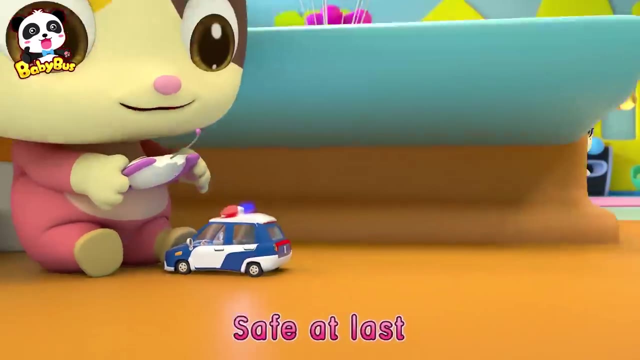 Run away, doo-doo-doo-doo, Run away, doo-doo-doo-doo, Run away, doo-doo-doo-doo, Run away. Safe at last. do-do-do-do-do, It's the end, do-do-do-do-do.